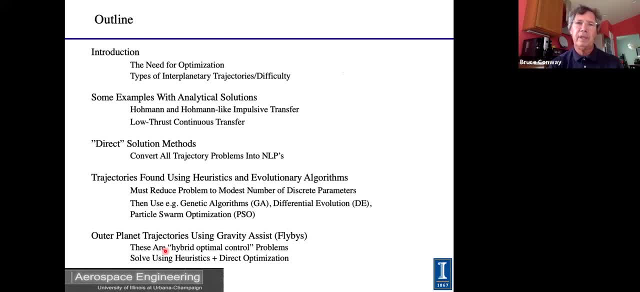 optimization is important- and then categorize the different types of interplanetary trajectories, which can be categorized by the difficulty of finding the trajectory solutions. I'll give you a couple of examples of cases where analytical solutions are actually available, and then we'll talk about the more interesting case. 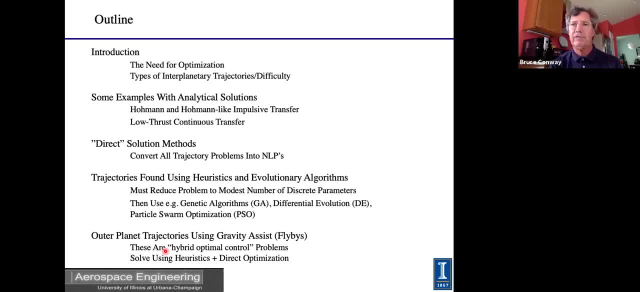 where the analytical solution is not possible and we have to use some more sophisticated methods to find trajectories. These are methods that have mostly been developed since about the 1980s. In fact, it pretty much spans my- by coincidence, kind of spans my- career as a researcher. 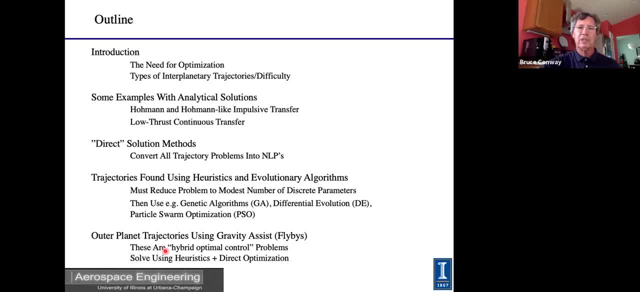 They're frequently called direct solution methods, as opposed to calculus of variations methods, which are referred to as indirect methods. Then we'll talk about probably the most exciting area right now in terms of trajectory optimization, which is the use of heuristic methods and evolutionary algorithms. 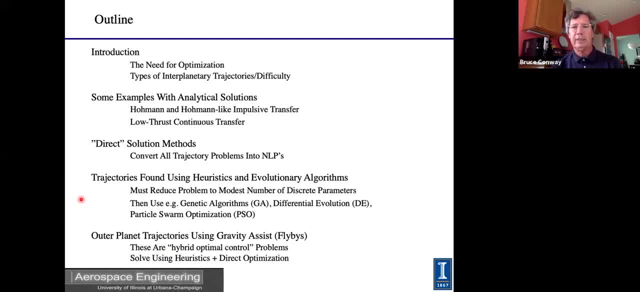 and I'll describe a little bit about what those are and why they, what advantages they have over some of the extent methods, and then I'll talk about some examples of using heuristic and evolutionary algorithms to find optimal trajectories. And then, finally, we'll talk about 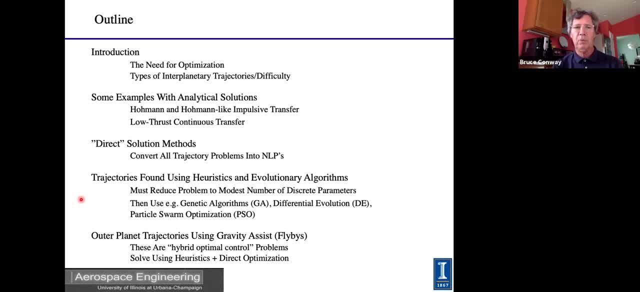 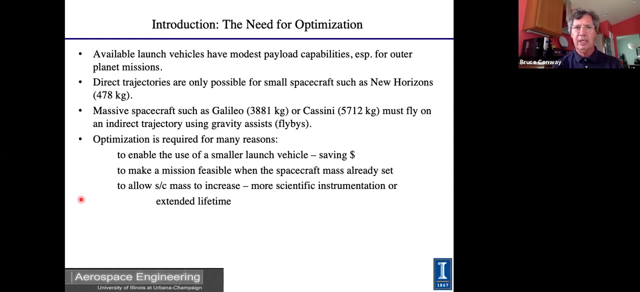 the most challenging problem, but a very practical one, of finding optimal outer planet trajectories using gravity assist fly-bys, that is to say, the kind of trajectory that was used for Galileo and then later Cassini and Krier. so why do we need optimization? well, we need it primarily because our technology with regard to 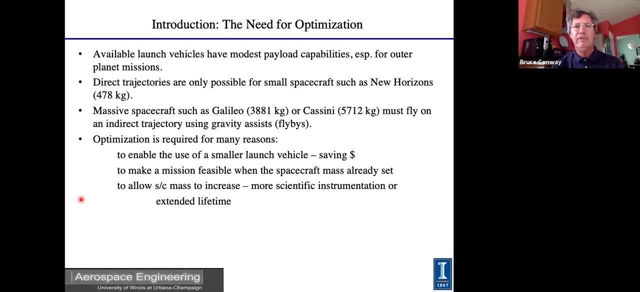 launch vehicles really is not very advanced. even some of our largest launch vehicles are not really all that capable, especially for outer planet missions. in fact, the only case that i know of where a direct trajectory was used for an outer planet mission was new horizons to pluto, but that 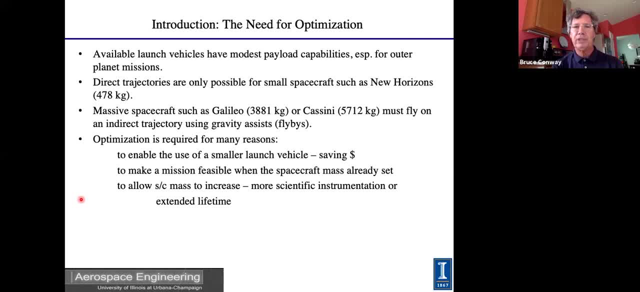 was a pretty small spacecraft. when you get to a spacecraft like galileo or cassini that are as as big as an automobile or or heavier um, the only way to do that with existing launch vehicles is to use uh, gravity assists or flybys. so you we need optimization. 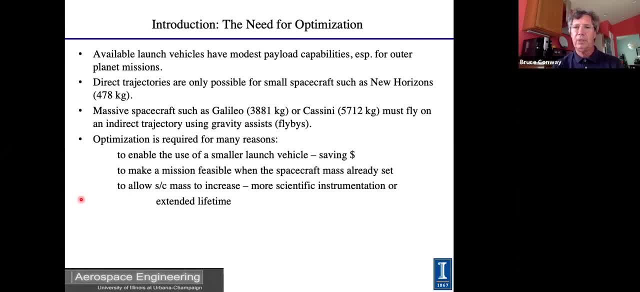 to do that with existing launch vehicles is to use uh, gravity assists or flybys. for many reasons, the technology that we have available is not that great. if you can optimize the trajectory, you might be able to use a smaller launch vehicle, and it turns out that roughly 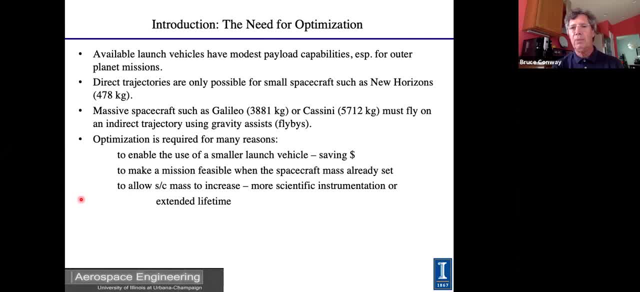 speaking, the cost of a launch vehicle is almost linearly proportional to its mass. so when you go from a delta to an atlas 5, to a spacex, uh, the, the heavy version, and so on, the, the cost is is roughly proportional to the size of the launch vehicle. so if, if nasa gives you a certain budget. 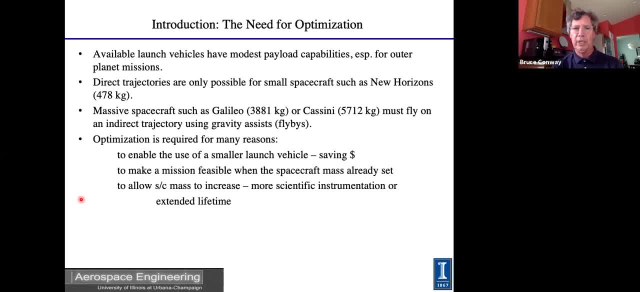 a lot of that budget goes to the launch vehicle. you'd like to use a smaller one, as you can. another important feature is to be able to, when you optimize, you can, trade fuel that you might otherwise have to use for scientific payload, and the scientists, of course, would like. 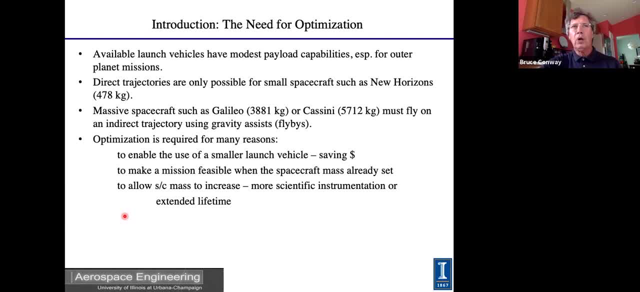 to increase the scientific payload, or you can use that fuel. rather than using it for the interplanetary trajectory, you can save it for using it in maneuvers around jupiter or around saturn and extend the spacecraft lifetime. so either way, if you can use less fuel for the 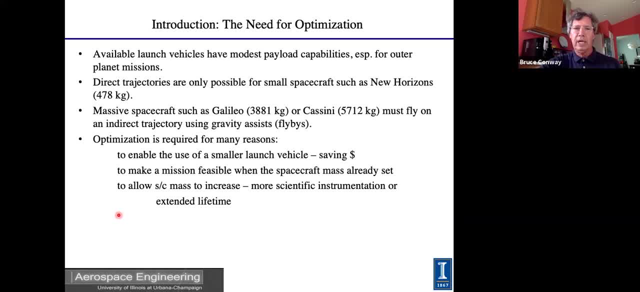 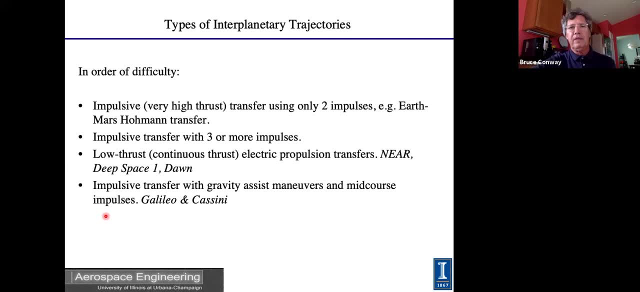 interplanetary trajectory? uh, you can. you can have a better scientific return or a longer lifetime. so the types of interplanetary trajectories, roughly in order of difficulty, very easy to find: impulsive, meaning high thrust, chemical propulsion transfer with just two impulses um, that could be, for example, an earth to mars homon transfer, even impulsive transfer with 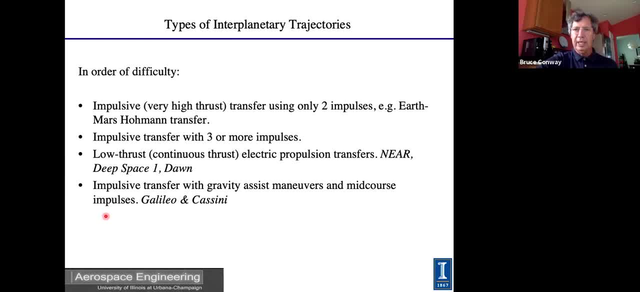 three or a small number more impulses is not too difficult to to solve for. but then a considerably more difficult case is that of low thrust, sometimes called continuous thrust, electric propulsion transfer. that would be exemplified by a spacecraft like near uh deep space, one which in fact, in 1998 was the first one to use that technology. 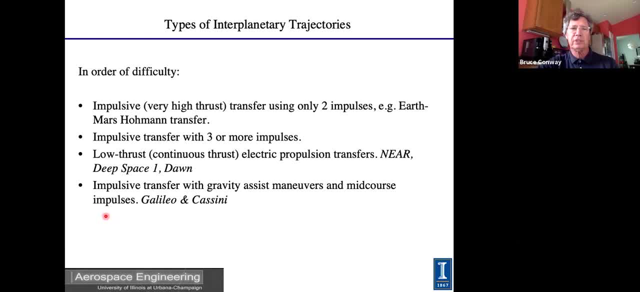 or the dawn spacecraft- i'm sure you're familiar with all those missions. um, when we say low thrust, we mean really, really low thrust. um, you're probably aware that something like the space shuttle main engine has a thrust that's measured at around uh 250 000 pounds of thrust, while the 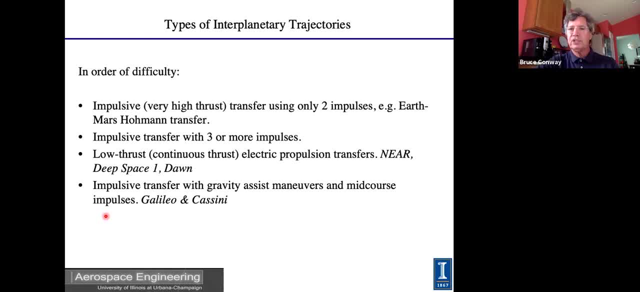 electric thruster is like the one on near: the thrust is measured in ounces, but when you're in field free space, remember that delta v equals a acceleration times, delta t. so even though the acceleration is very small, it's down to maybe 10, to the minus 5 g, the burn time compared to the space shuttle. instead of 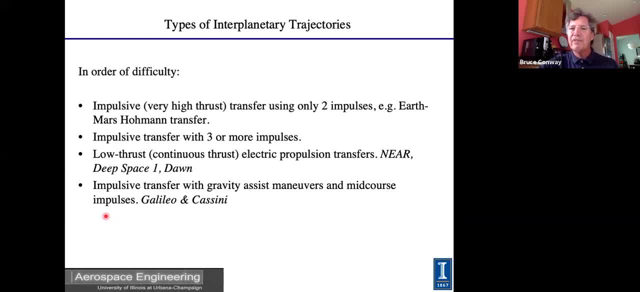 maybe 10 to the second, seconds goes to 10 to the fifth or 10 to the sixth. so the product of acceleration times, time, gets you to roughly the same final velocity as as the larger thrust engine. uh, and then, finally, the most difficult case to consider, well, maybe i shouldn't say most difficult. 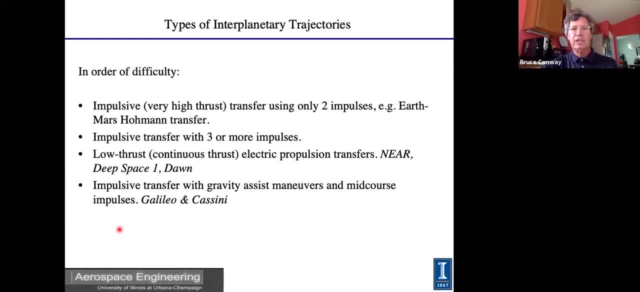 the most difficult we've done so far is impulsive chemical rocket transfer using gravity assist maneuvers and possibly some mid-course impulses. i could add what would be the very most difficult case, which would be low thrust transfer combined with gravity assist maneuvers, but i don't know of 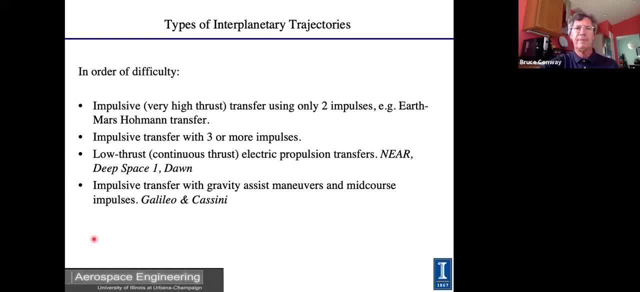 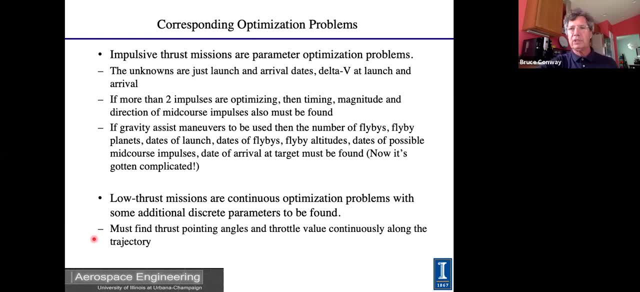 any that we've done yet so far. So impulsive thrust missions are relatively simple to solve because they're just parameter optimization problems. So you need to know the launch and arrival dates- the delta V at launch and the delta V at arrival- If you're going to use more than two impulses. 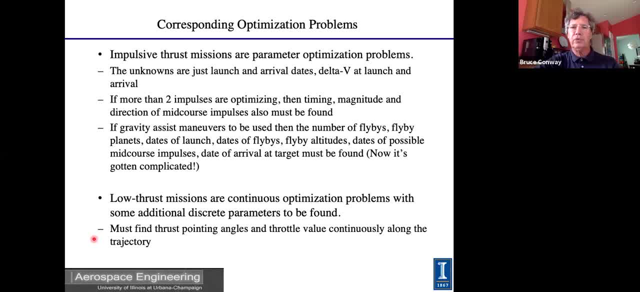 then you have to find out where and when to do the mid-course impulse. That adds a little bit of complication. On the other hand, if you're going to use gravity assist maneuvers, then it becomes much more complicated. Then the number of flybys, the planets you're going to use for flybys, 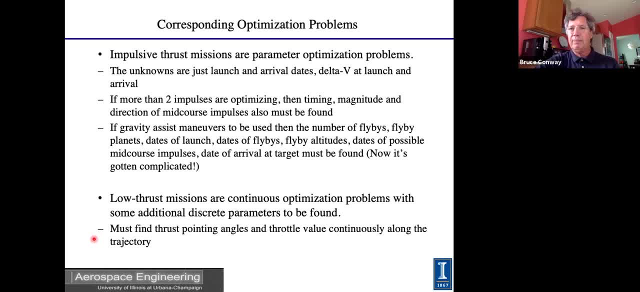 the date of spacecraft launch, the dates of the flybys, the altitudes of the flybys, the dates and timing of or the timing of the launch. the date of the launch. the altitudes of the flybys. 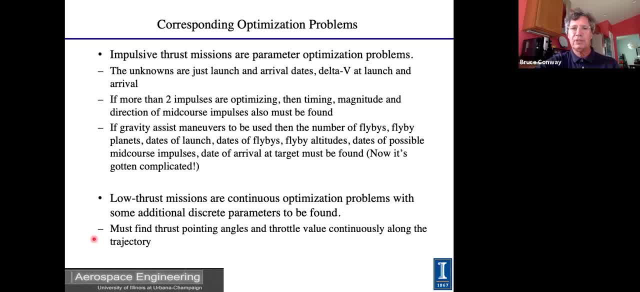 and direction and magnitude of possible mid-course impulses, the date of arrival at the target, all those things have to be found, And then that becomes a quite complicated parameter optimization problem. On the other hand, low-thrust missions are continuous optimization problems. They usually only have a small number of discrete parameters, such as the: 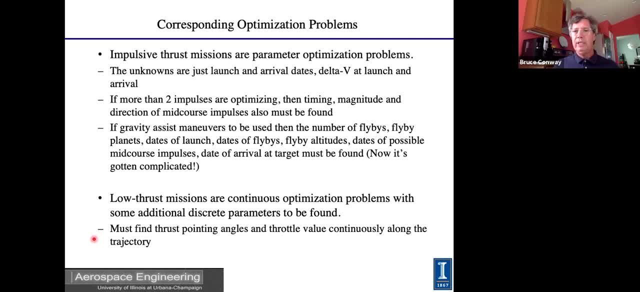 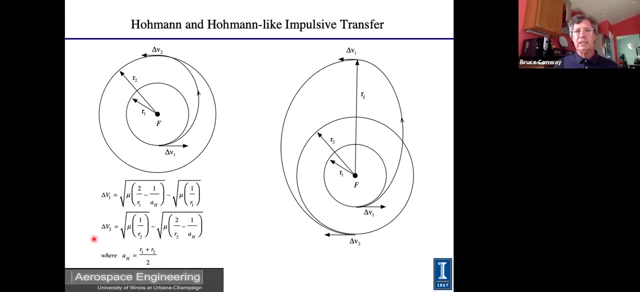 launch date and the arrival date, And then in between you need to find a continuous history for things like the throttling parameter, meaning the thrust that you're using and the thrust pointing angle. So here's the simplest case, And many of you have probably seen this in elementary. physics, or maybe you've taken an orbital mechanics course- Hohmann transfer. Why is that relevant? Well, it's relevant because most of the planets that we go to are in nearly circular orbits, Mars being a bit of an exception, But even there you can. 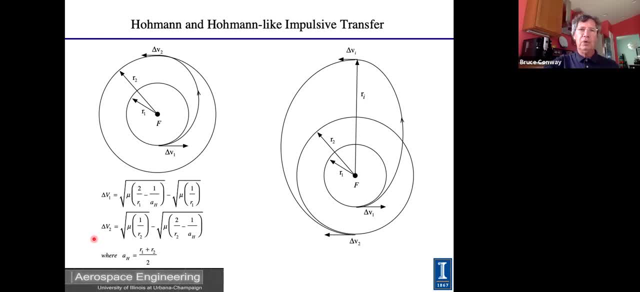 use something that's like a Hohmann transfer. So I've shown the Hohmann transfer in this left cartoon going from a circular to circular orbit. The transfer orbit has a periapsis at the initial radius and apoapsis at the final radius And the periapsis at the initial radius and the periapsis. 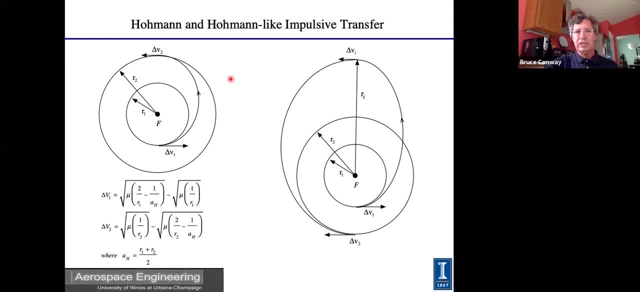 at the final radius and the periapsis at the final radius and the periapsis at the initial radius and the periapsis at the final radius. the velocities are parallel to the existing velocity. It's very easy to calculate the two delta b's with this formula. Now, this is for a. 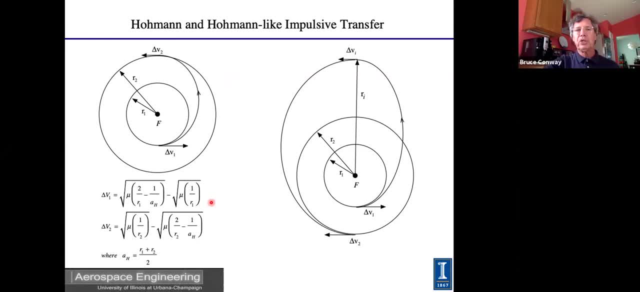 coplanar case. Even if it's a three-dimensional case, with inclination changes at each of the two burns, that's still very easy to solve. It just becomes a. there's a vector triangle and you have to find the third side using the cosine law. 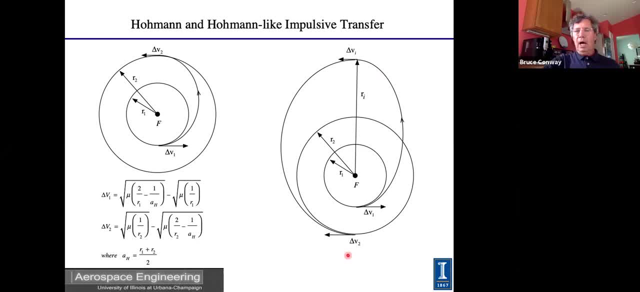 It's still very easy. What I call a Hohmann-like impulsive transfer is this one on the right-hand side. This actually has a name. This is called the bi-elliptic. It's a three-impulse transfer. 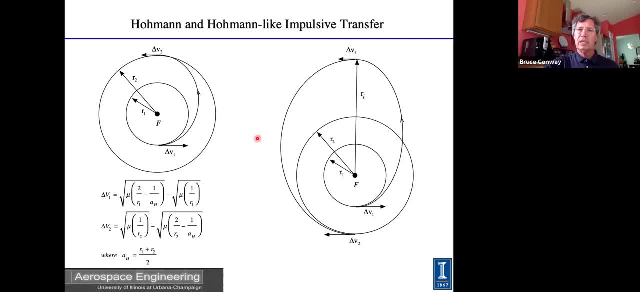 This can actually be optimizing in some circumstances, especially if there's a very large inclination change to be done, because that inclination change is almost exclusively done out at this distant point where the burn is not going to be able to be done. So 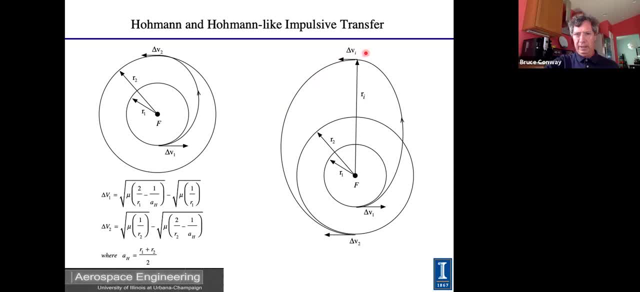 the velocity is small because the spacecraft has traded kinetic energy for potential. sorry, it's traded kinetic energy for potential energy. So a inclination change, plane change maneuver is very cheap out here and that can make this kind of transfer optimizing. 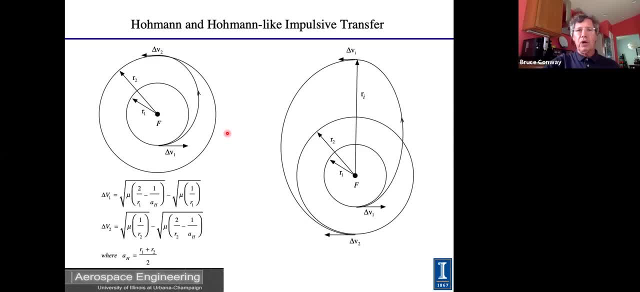 If you, oh, let me just say so, the Hohmann is easy to calculate and in fact, there are three spacecraft that are almost at Mars, going to be there within the next week, that have used Hohmann transfer. And of course, the Hohmann transfer requires. 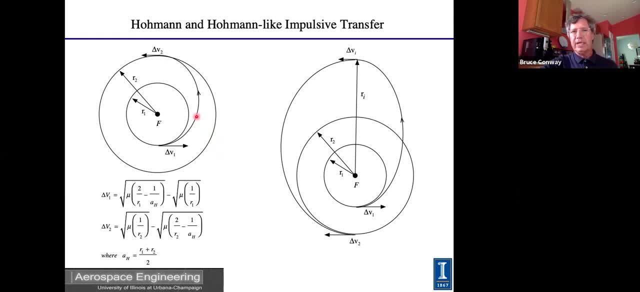 that the target planet, let's say in this case Mars, has to be at a particular point on its orbit here- outer orbit- at the instant that you leave the Earth, so that, as the spacecraft moves toward Mars, Mars is probably going to be able to move to the other side of the planet. 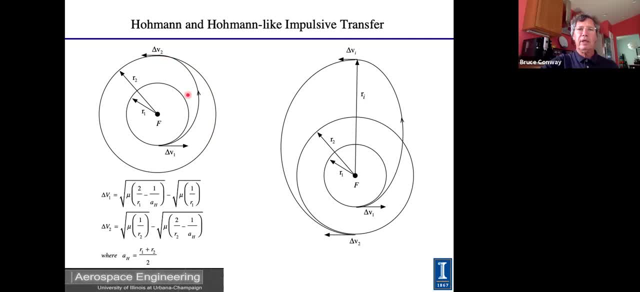 Mars is going to meet it at this point. That lead angle is about 44 degrees, by which Mars has to lead Earth, and that occurs every 26 months, and so if you look at the history of Mars missions, you'll see that they take 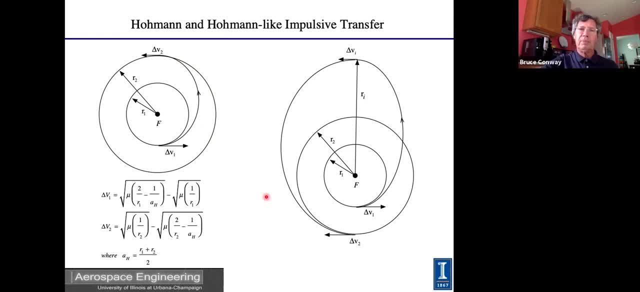 advantage of the Hohmann transfer and um launch about every 26 months And a back of the envelope kind of calculation of the delta-v required, We'll probably get get you within a couple of percent of the actual delta v. of course it's ignoring things like the. 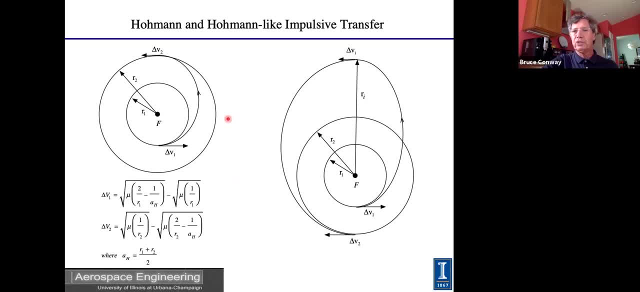 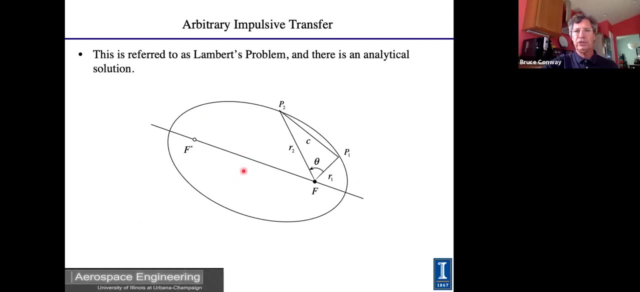 gravity of other planets, solar radiation pressure and so on, but those are relatively small and and it's reasonable to assume that the spacecraft is moving on a keplerian ellipse. so you you can do a very good back of the envelope calculation of the velocity change required. if you aren't able, 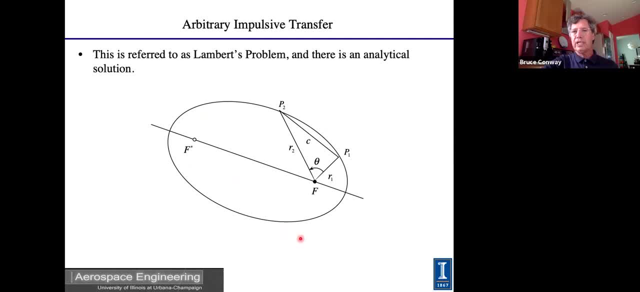 to do a homon transfer, that is to say a transfer through 180 degrees. there's still an analytical solution. suppose that point p1 here is the position of earth at departure. p2 will be the position of mars when you want to arrive. so you know the radius vectors, you know this interior. 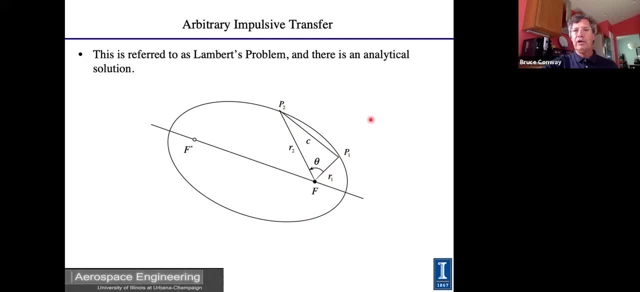 angle and so on. if you choose a desired flight time, which of course you have to know if you you are going to determine where the planets are at launch and and arrival. if you choose the flight time, then the problem is to find a section of an ellipse that joins these two points. 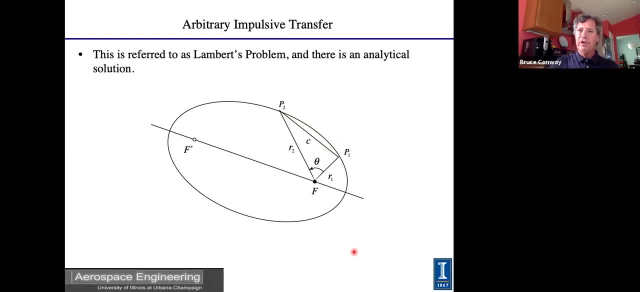 in the uh required flight time. that's referred to as lambert's problem, and there's uh that can be solved analytically. um, even if you have uh plane change maneuvers as part of it, and um, it's very well described in this textbook that siegfried mentioned that one of my colleagues and i wrote. 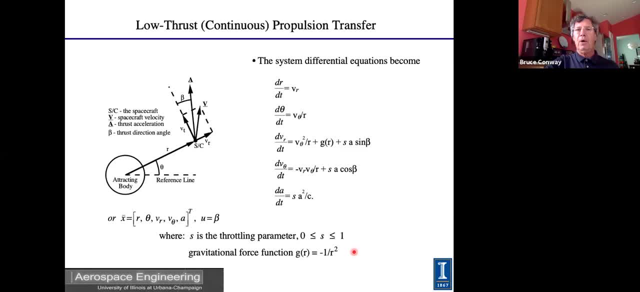 it's called orbital mechanics. okay, so the impulsive cases are relatively straightforward. what about the low thrust case? well, that's a qualitatively different problem. we can no longer assume that the spacecraft is on a keplerian elliptical trajectory. it is at any instant, but 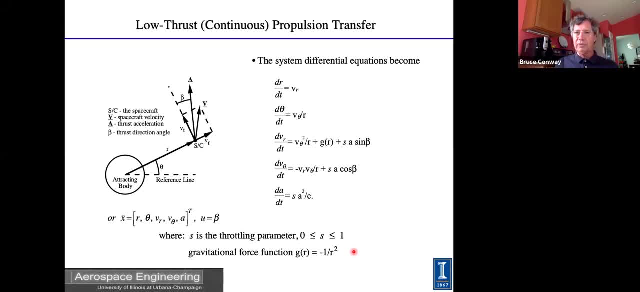 the precise ellipse is on a keplerian elliptical trajectory, so we can no longer assume that the ellipse is always changing because of the thrust. so in two-dimensional polar coordinates- here the system differential equations- notice that the thrust comes in on the right hand side of these. 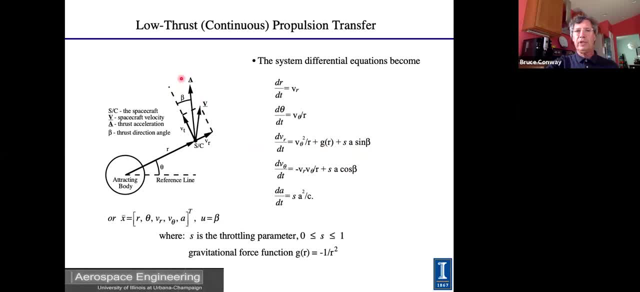 two equations. beta is the thrust pointing angle that you can see here. beta would be zero if the radial component of the thrust is zero. a is the maximum available acceleration and s is a throttling parameter. that simply is a number between zero and one. now notice the fifth equation. this is the time rate of change of the maximum possible acceleration. 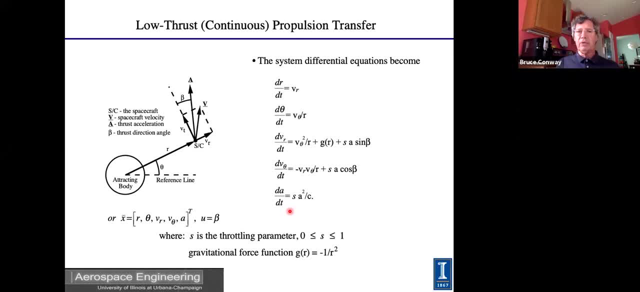 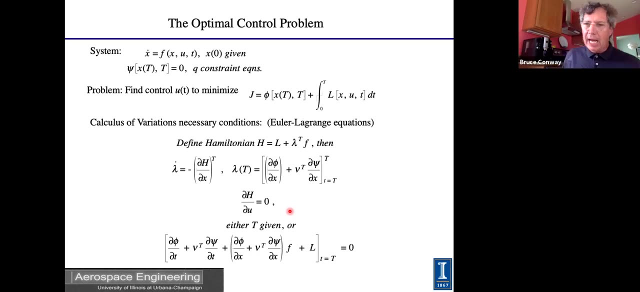 and the reason that that is in there is because that acceleration increases as fuel is consumed. uh, an equation for d, mass dt would do just as well. so how do we find a minimum fuel trajectory for a system governed by that set of first order ode's? well, that was figured out 200 years ago by very eminent mathematicians. 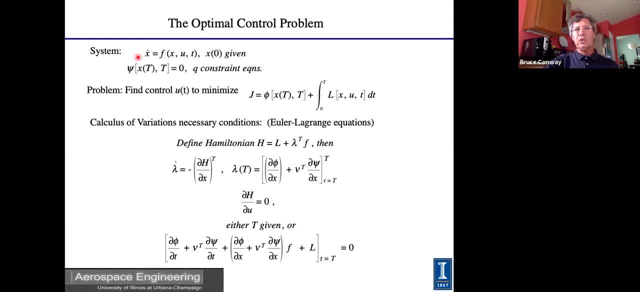 let's let this quantity x doesn't look like a vector, but let's let it represent that five element state vector that you saw on the previous slide. so you represent a vector of the control variables, in this case the thrust pointing angle. so it's a scalar. and suppose that we have a set of q constraints that are functions of the states. 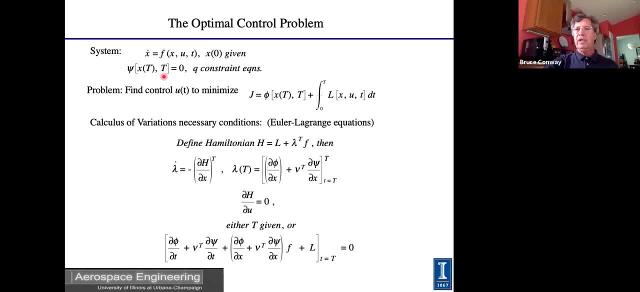 at the final time, and possibly the final time itself. these could be as simple as saying that the position and velocity, the r theta, vr and v? theta of the spacecraft need to be equal to that of mars at the final time, whatever that final time is. so you might have four simple constraints. 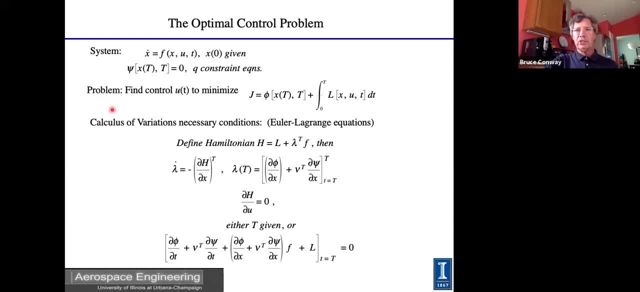 so we want to find the control time history that minimizes this function. this is the usual choice for the cost function it's. it combines a function of the final states and the final time, this quantity, capital t, with an integrated history of the states and the controls from the beginning to the end of the trajectory. 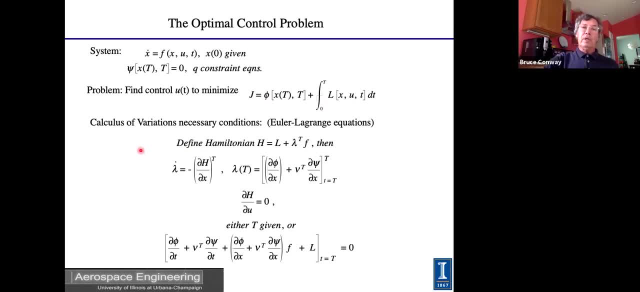 so the necessary conditions for a minimum of j are the calculus of variations, necessary conditions referred to as the euler-lagrange equations. we define what's called the hamiltonian, which is the integrand of the cost function plus the right hand side of the. in this case, 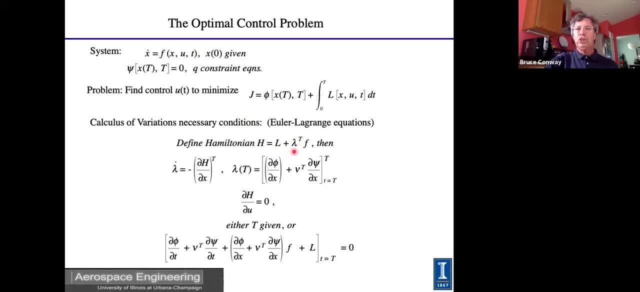 five system differential equations, adjoined through a set of costate variables, this vector lambda. they're called costate variables or continuous lagrange multiplier variables. i'm sure you're at least familiar with lagrange multipliers. for the discrete case, here they're continuous variables, and so the necessary conditions become, of course, these two conditions, this satisfaction. 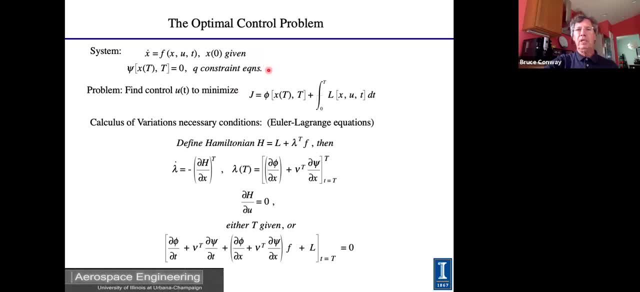 groups and Boolean and NiE and allen terms that exist here in this particular equation that we often call � 결과 pictures express the separation equation of the differential equations of motion the terminal constraint equations then we have to add differential equations for the diaper Hamiltonian with the control variables has to be equal to zero. And then either the final time 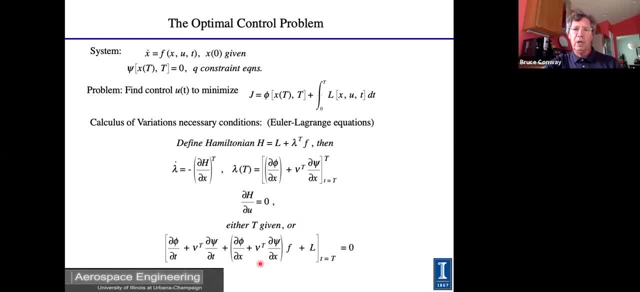 is specified, or you can add this scalar equation that has to be satisfied at the final time and allows you to find out what the optimal final time is. So notice what we've done. We've taken a system of what was originally five ordinary differential equations And we've now made it. 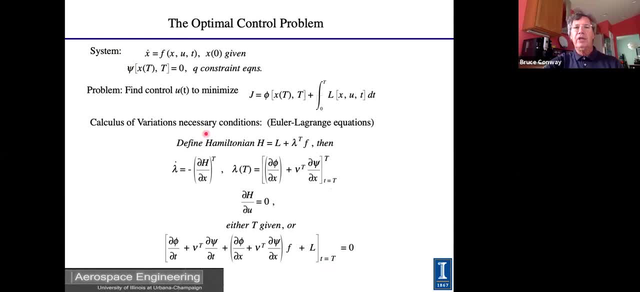 a system of 10 ordinary differential equations. The original system has initial conditions specified. The new system has some of the initial conditions given at the starting time and other conditions given at the final time. So this is referred to, as you probably know, as a two-point. 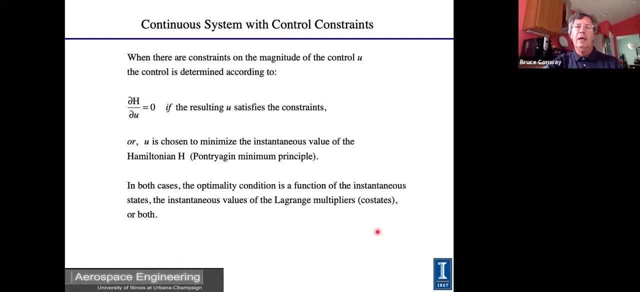 boundary value Problem. Now, another complication is that we often can't use this optimality condition- dH, du equal to zero- to solve for the optimal control. That happens in a number of circumstances. One is when the Hamiltonian is linear in u And so. 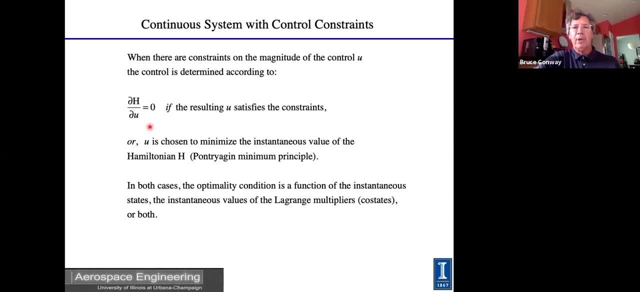 this equation doesn't give you any useful information. But another case is if the optimality condition, even if it's a two-point boundary, it's not a two-point boundary If it works- gives you a? u that is not within the available bounds for you, And this happens all the. 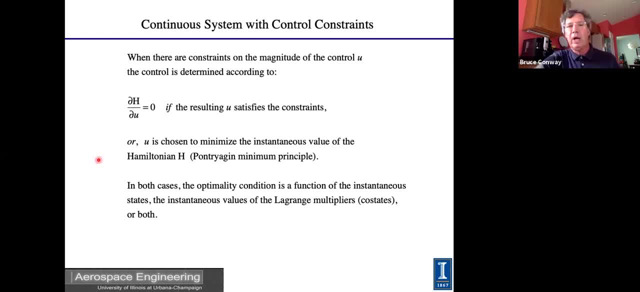 time. For example, in the spacecraft case, if you want to minimize flight time, this would tell you to use infinite thrust. You don't have infinite thrust, You have an upper bound. So in that circumstance we replace that condition with what's called the Pontryagin minimum principle. 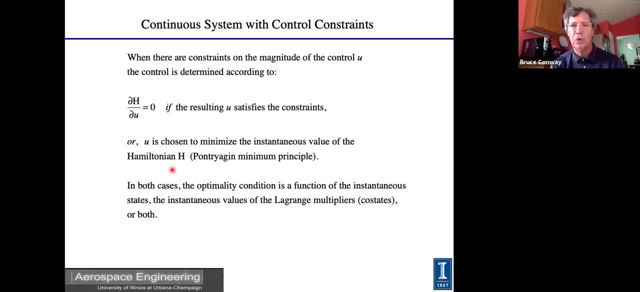 which says that the instantaneous value of the optimal control is. the value of the optimal control Is the one that instantaneously minimizes the Hamiltonian over all possible values of? u Somebody at the front door, That's the dachshund. Okay, So just to give you an example for this: 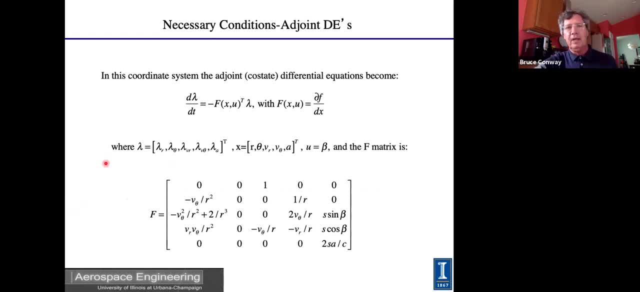 particular relatively simple problem. the differential equations for the costate variables are given by this equation And the F matrix that you see in there is. the differential equation for the costate variables is this: So you can see that the differential equations for the costates are linear in the 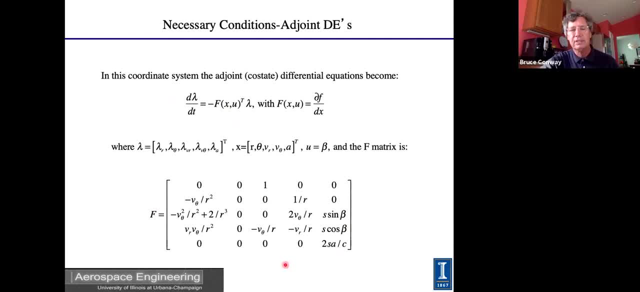 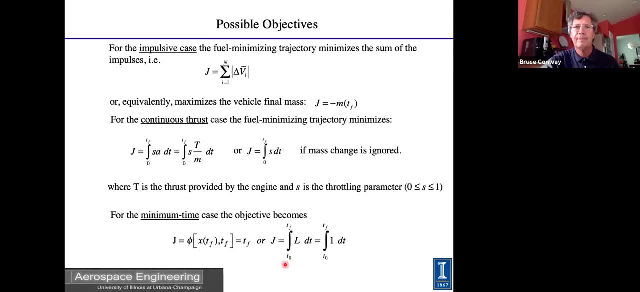 costate variables but non-linear in the states. So we've significantly complicated the problem. but there's no way to avoid that Now, as far as possible, objectives. in the impulsive case, usually the easiest thing to do is to maximize the vehicle final mass, which means that you've 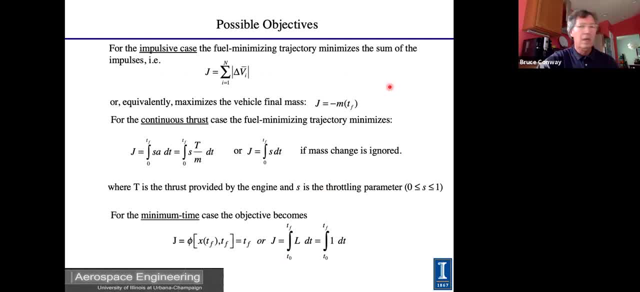 minimized the propellant used. Come here So to do that. we want to minimize the negative of the final mass, so you maximize the final mass In the continuous thrust case. usually the easiest thing to do the fuel minimizing trajectory is to let the integrand 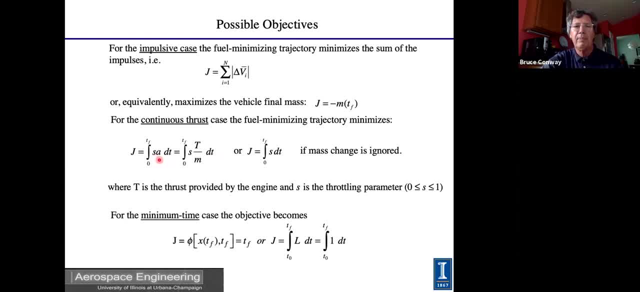 this capital L function be the throttling parameter times the acceleration, So effectively integrating that over time, integrating the acceleration gives you the delta V. And remember the rocket equation, sometimes called the Tsiolkovsky equation, that says that the propellant mass required 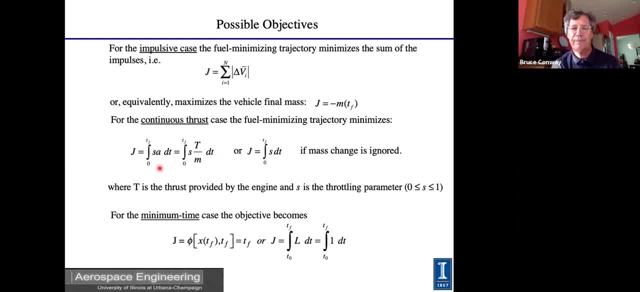 monotonically increases with the delta V. On the other hand, if you want to do a minimum time case, which sometimes arises, the person writing the the equations can either choose to let this function of the final time simply be the final time, or you can let that phi function be zero and let the integrand in the cost function simply be. 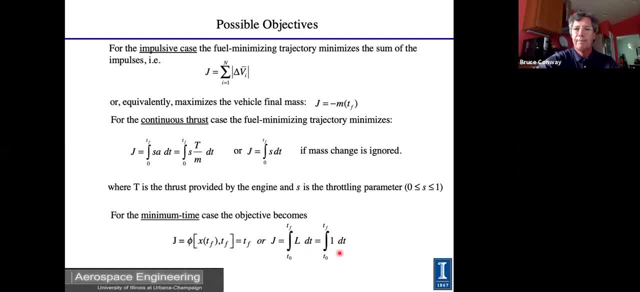 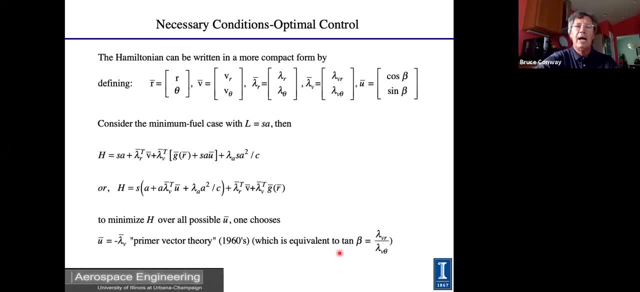 one, So integral one. dt is delta t. You get the same. you have to get the same solution either way. Now let's write the Hamiltonian in a little more compact form By forming these vectors: one for position, one for velocity, one for co-states corresponding to: 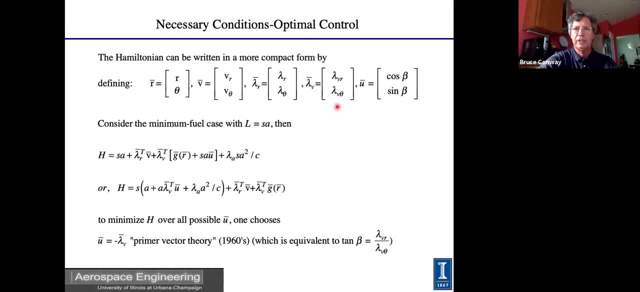 the position coordinates and one for co-states corresponding to the velocity coordinates, and let u be represented by the cosine and the sine of the thrust pointing angle. Then, if we use a minimum fuel case with this cost function that I showed you on the previous slide, 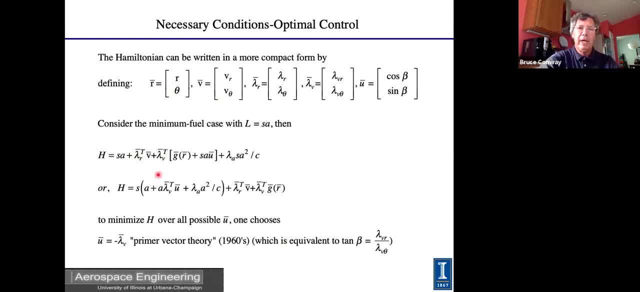 this is the new Hamiltonian, And if I rewrite that to isolate the throttle parameter, you get this expression. And now if I apply Pontryagin's minimum principle to minimize h over all the possible u's, well, u appears in only one place right there. So to minimize the 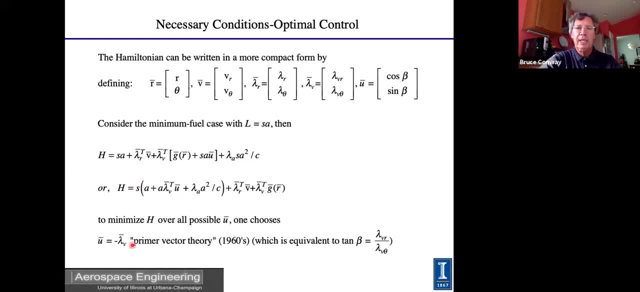 Hamiltonian, what I do is I choose u to be in the opposite direction from lambda, from the lambda V, which is this vector up here. That makes this as negative as possible, And one can show without much difficulty at all that what that implies then is that the optimal. 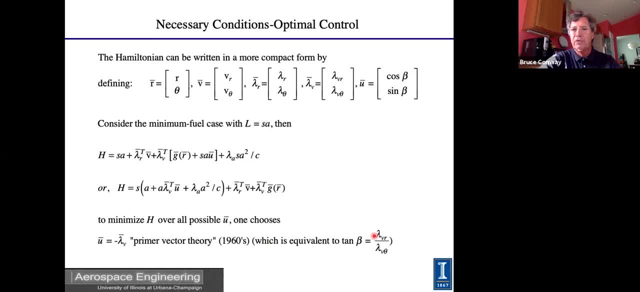 thrust pointing angle. beta is the arctangent of the ratio of one of these co-state variables over the other, the lambda VR over the lambda V theta. So what's this mean? It means that if you can solve the two-point boundary value problem, 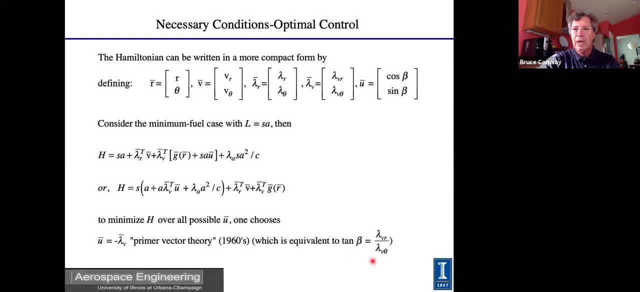 then this expression right here. you will then have lambda VR and lambda V theta, known as functions of time, from the starting time to the ending time, And so, at any point in time, you can evaluate what the optimal thrust pointing angle is. Now, how about the throttling parameter? 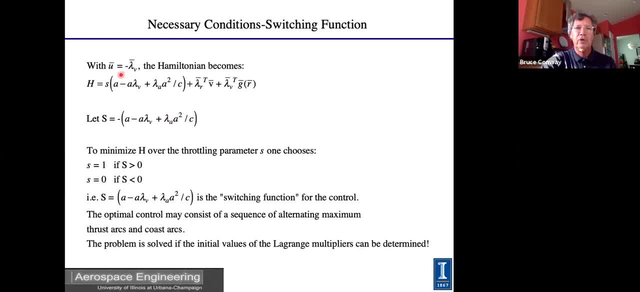 Well, this is just if I let you be the negative of the lambda V. here's the Hamiltonian, And now the question is: what's the optimal value of the throttle parameter? Well, suppose we define what we call the switching function as the negative of this quantity that multiplies the throttle parameter. 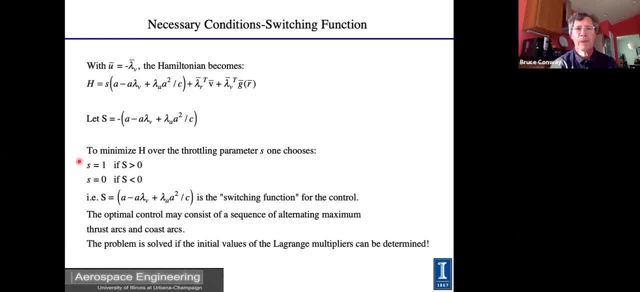 Then you can see that to minimize the Hamiltonian, what you want to do is you want to use maximum parameters, Maximum thrust if this quantity is positive and no thrust if that quantity is negative. For this simple problem, this, arises a lot. 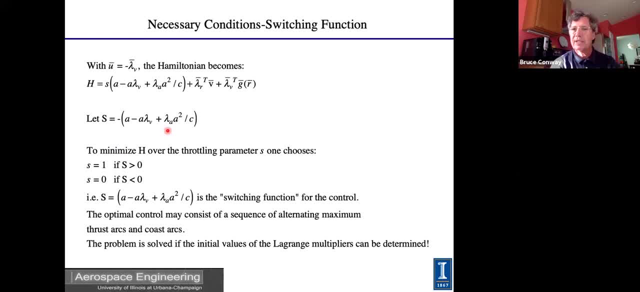 There is no case where intermediate thrust is minimizing, So the throttle is either fully open or fully closed, And in fact an optimal control can consist of a sequence of alternating maximum thrust arcs and co-scales, So that switching function can then be found as a function of time. 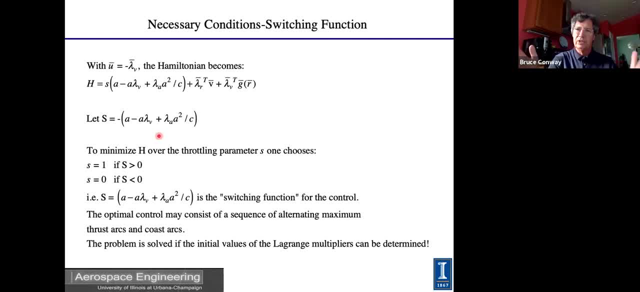 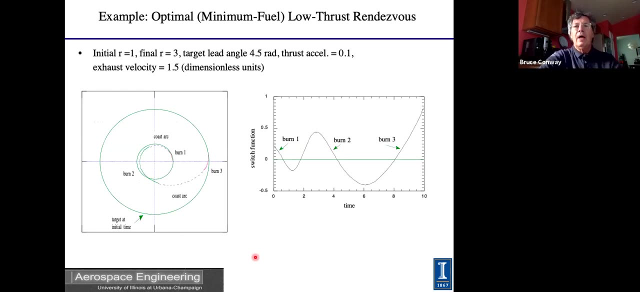 if we've solved the two-point boundary value problem from the starting point to the ending point. So we get everything we need to know. The only problem is what are the initial values of the Lagrange multipliers? So here's a simple example. 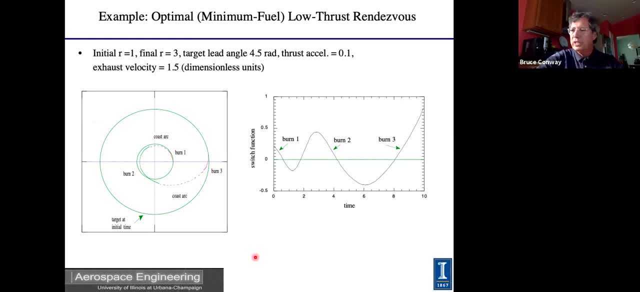 This is one of the first ones that we solved this way A long time ago, So it's a typical problem. This is a minimum fuel, low thrust rendezvous. There's a spacecraft that's in this orbit at 1 AU and we want to get out to 3 AU and rendezvous with a target that starts here. 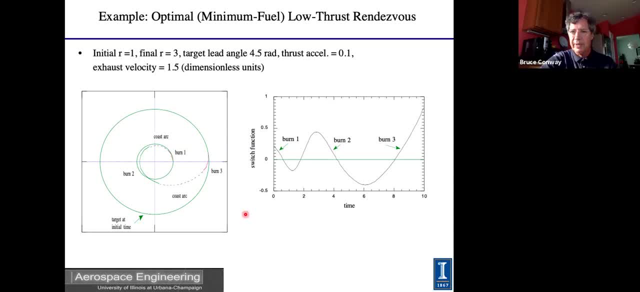 And it turns out that if you solve this problem using just the method I described, here's the optimal solution: There's a burn because the switch function is positive to this point, then it coasts, Then there's a burn, then there's a longer coast and then there's a final burn. 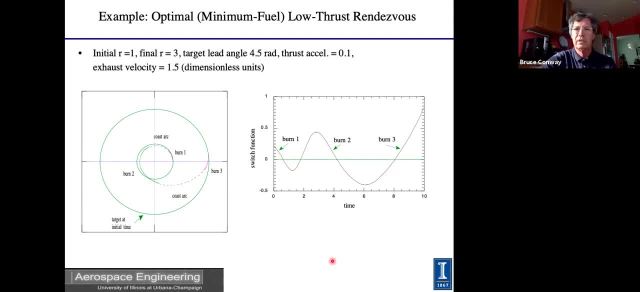 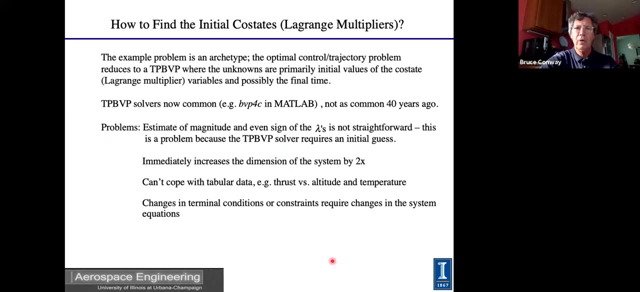 And this is relatively straightforward to solve if you have a good two-point boundary value problem solver. But this is a fairly simple problem. It's not even terribly extremely challenging for a two-point boundary value problem solver. that's in MATLAB, Okay. So what's the difficulty of using this approach? 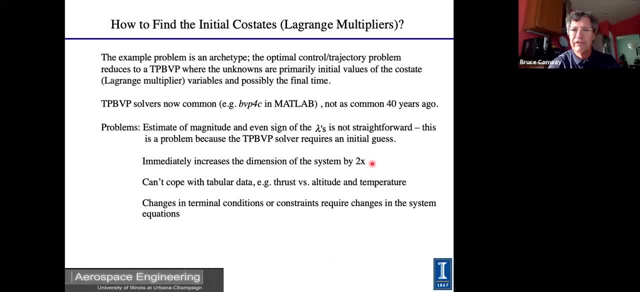 Well, as you saw, it makes the system bigger. Instead of five differential equations, we have 10.. I'm going to skip a couple of these. The other main problem is that every two-point boundary value problem solver. some of you probably had experience with this. 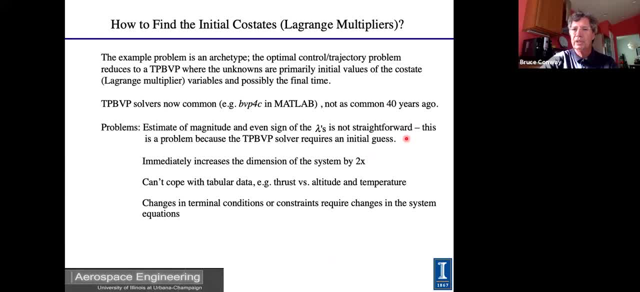 it needs to be given an initial guess of the solution, And you may not have that. If you don't give it a good enough initial guess, it simply won't converge. Or if you could give it an initial guess, the other thing that can happen is it will converge to a solution that's in the neighborhood of the initial guess. 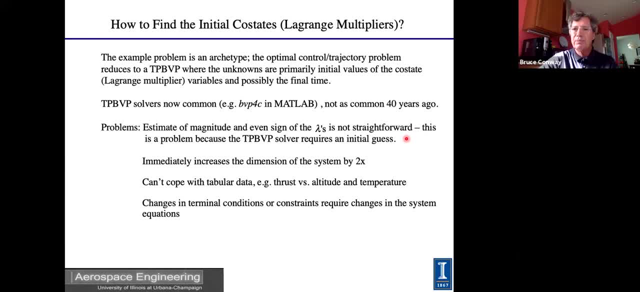 Now the difficulty with that is that many of these problems have lots of local minima. obviously only one global minimum, But the necessary conditions are entirely satisfied by the local minima And you won't know that you have found a local minimum. 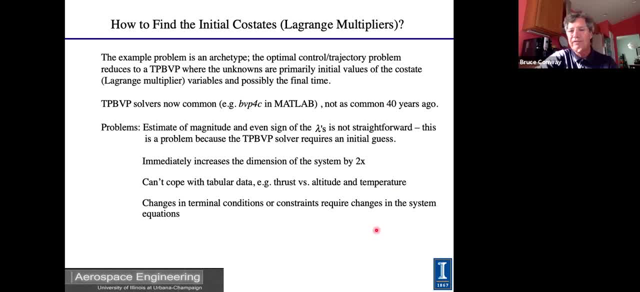 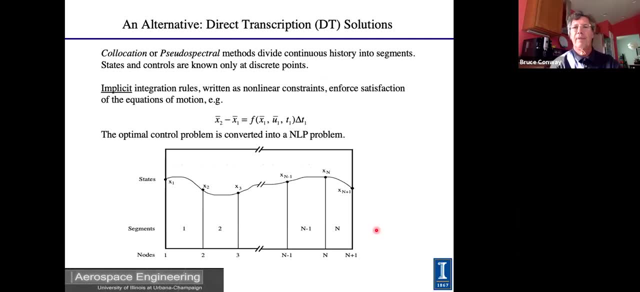 Okay, There's no feedback to tell you that. oh, you only found the local minimum. There's a better minimum out there, Okay. So as an alternative to this problem of solving two-point boundary value problems, in the early 1980s a new method was found. 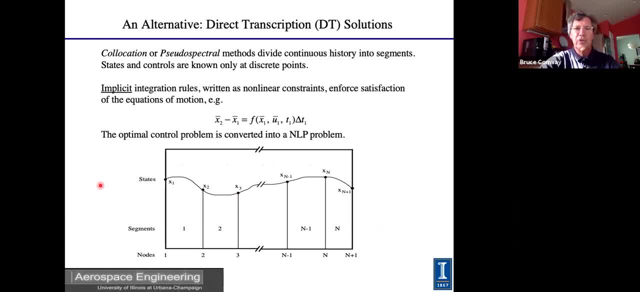 It's called direct transcription solution. So the basic idea here is in this cartoon. suppose this is just one state, could be the R quantity or the theta quantity. We assume that it has a certain continuous time history And we discretize the time into N segments. 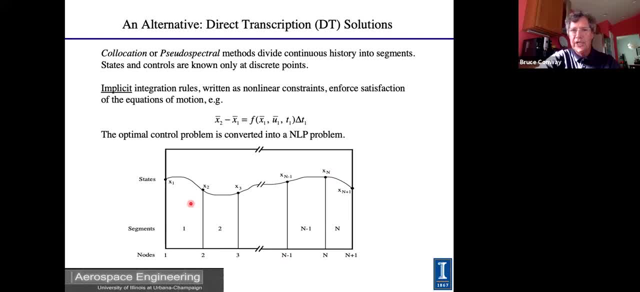 There would be a similar cartoon for the other four state variables and a similar cartoon for the one control variable, the thrust pointing angle. Then the states at these discrete points become parameters in a non-linear programming problem solver. But they're not arbitrary because they have to satisfy the system differential equations. 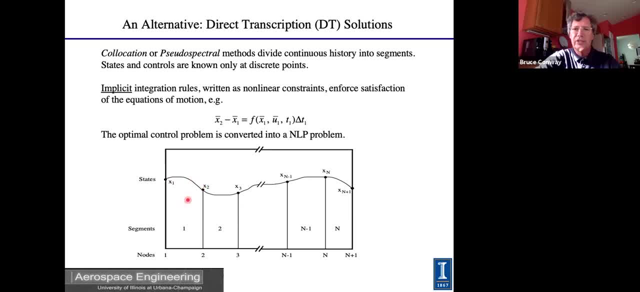 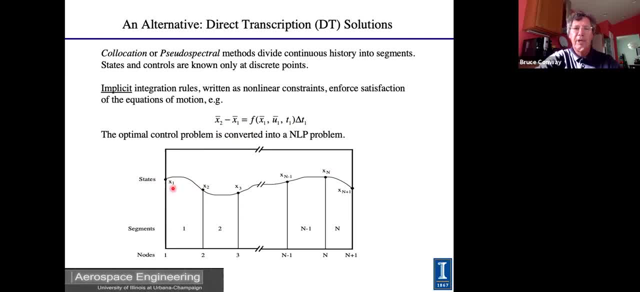 evaluated at X1 times Delta T. Well, that would be a very poor approximation for this case, because F evaluated here looks like the slope at this point and it would put you up here when you really want to be down here. But if you have a lot of segments between here and here, it would work. 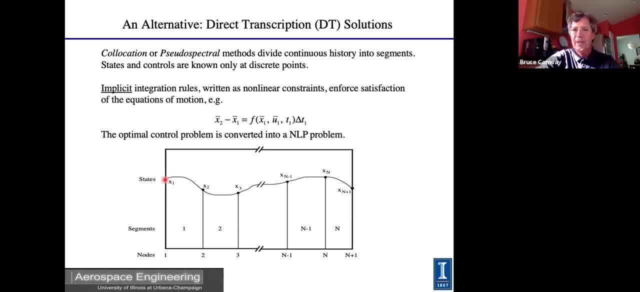 If it's just a small time, it would not be a bad approximation. OK, so This becomes a non-linear programming problem. next, OK, so this becomes a non-linear programming problem. next, you want to minimize a certain function, such as final time or the negative of the final mass. 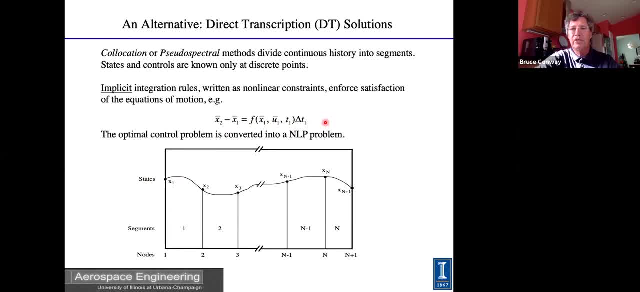 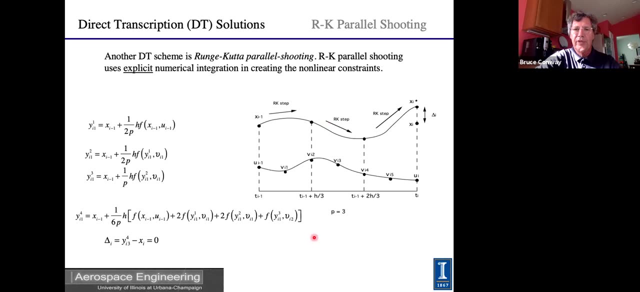 Putting in a whole bunch of constraints like this enforces satisfaction of the system, differential equations, and you also can input upper and lower bounds on the states and the control variables. Here's an alternative that we came up with in about the late 1980s that I like a little better. It's qualitatively similar. This would be just. 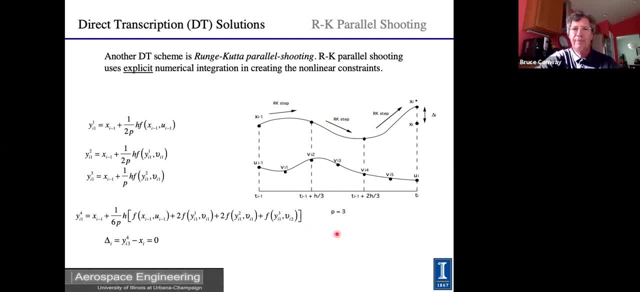 one of the segments that you saw in the previous cartoon. What we use now instead of a simple Euler step is Rk, is the four steps of an Rk parallel shooting. So suppose that the nonlinear programming solver thinks that one of the states has this value at the left-hand side of the segment. 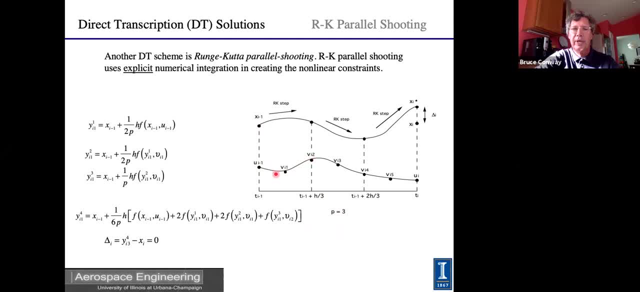 and you use these controls at these three points in the right-hand sides of the Rk step formulas and you propagate to here. Well, you get a value for the state. but let's not make it an NLP parameter, Let's just use that. 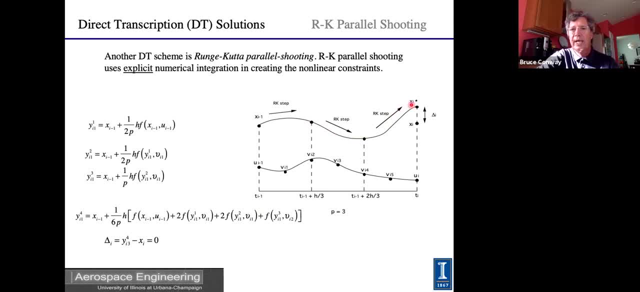 to initialize another Rk step and then do it again until you're all the way over here. Well, this value up here is what you get by using Rk integration, But the NLP solver thinks that the value is this, so you have to have the NLP solver close that gap. 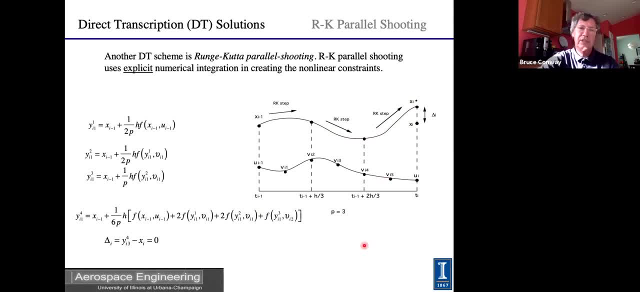 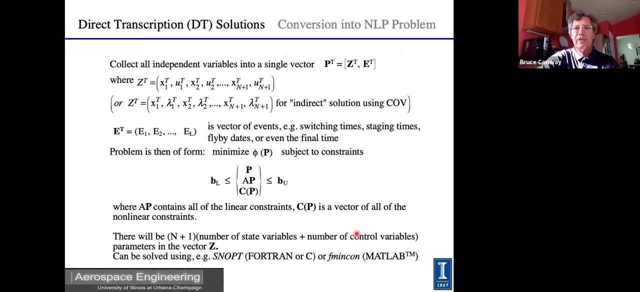 by forcing it equal to zero, And this actually works quite well. It has the virtue of minimizing the number of parameters that you need for the states, but using a lot more for the controls, which is generally a good thing. So this just describes the nonlinear program. You have a long 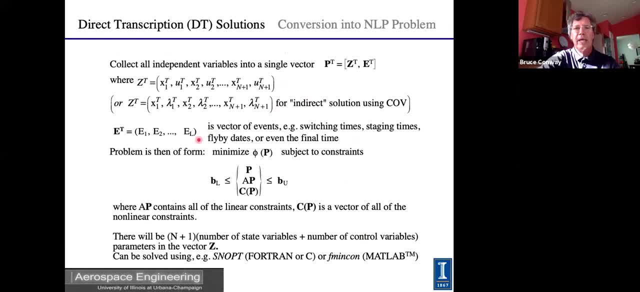 vector of all the states and all the controls. You may, in addition, have some discrete parameters, like a launch date or, if you're looking at solving a launch vehicle problem, maybe the staging times, An interplanetary trajectory problem. some discrete parameters could be fly-by. 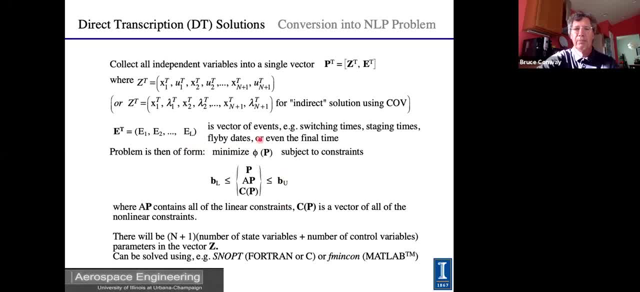 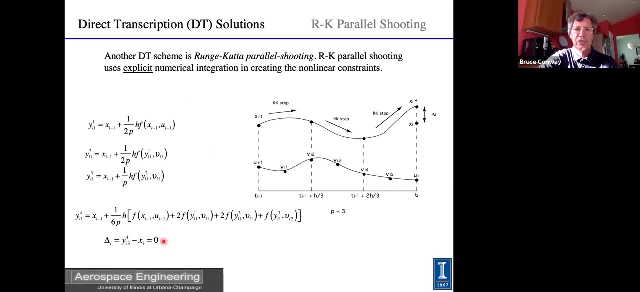 dates, etc. And so this is basically a nonlinear program. We have upper and lower bounds on the parameters themselves, the state variables, usually no linear bounds. but then the C of P is a collection of all the nonlinear constraints And if they are, this last step that closes the gap at the right-hand side. 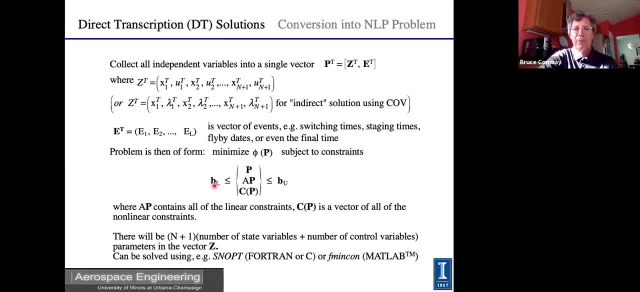 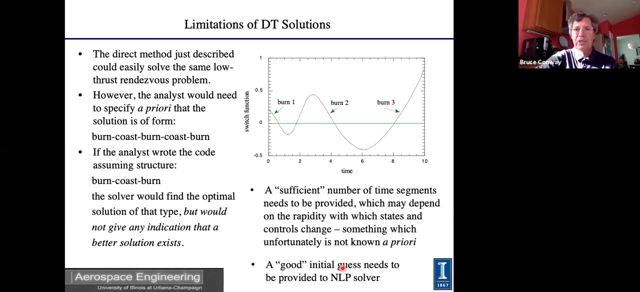 then the upper and lower bounds for that will be zero. And you can solve that kind of problem using, for example, fmincon in MATLAB, And we've solved problems with as many as 3,000 parameters, So you can do a fairly fine discretization of the time history. So that method would solve this. 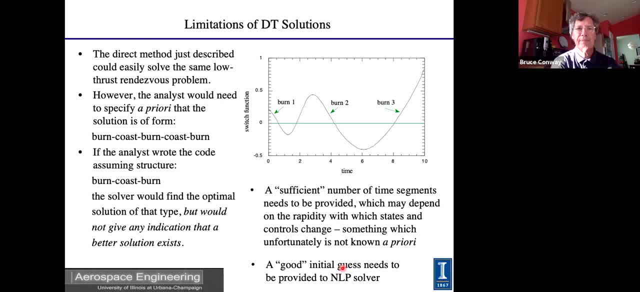 problem I showed you earlier very, very easily, But it has limitations. You have to specify a priori what the form of the solution is going to be And you have to specify a priori what the form of the solution, of the solution, is going to be. And you have to specify a priori what the form of the solution. 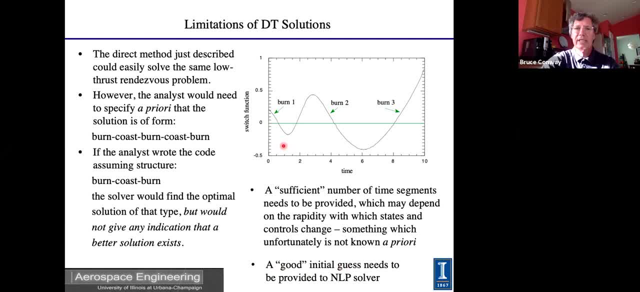 is going to be So in this case. if you tell it that the solution is what it actually turned out to be: burn, coast burn, coast burn- you'd get this solution. But what if you don't know that? 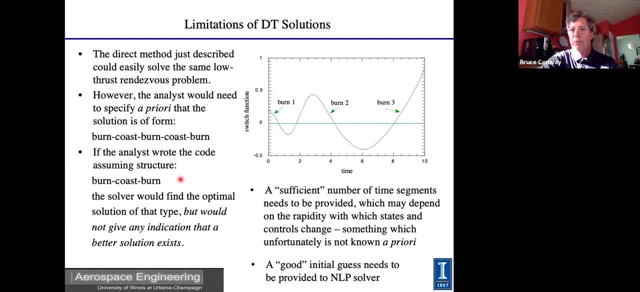 If you think that it's just going to be a burn coast burn kind of like a low-thrust Hohmann transfer, well, the solver would give you that. It would give you the optimal solution that has a burn coast burn structure, but it wouldn't give you any information that tells you you can do. 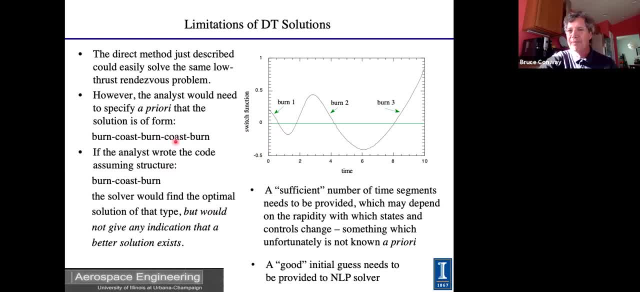 better if you add another burn and another coast, So you get what you asked for, which is a little bit of a problem, But you can avoid that in some cases by over-specifying. For example, I could put an initial coast in here ahead. I can make it: coast burn, coast burn, coast burn. 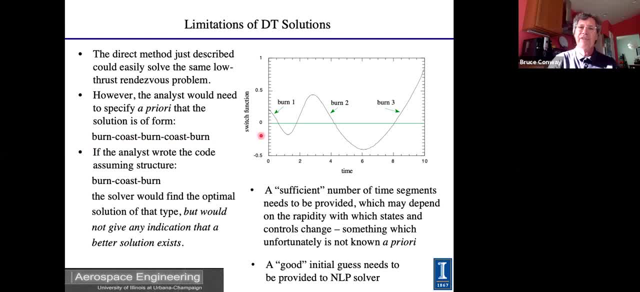 and then even add another coast and burn And if they are not not optimizing, they get collapsed as the NLP solver solves the problem. So you can over-specify and then you would get the right answer. But the big problem down here is that, just as with two-point boundary value problem solvers, 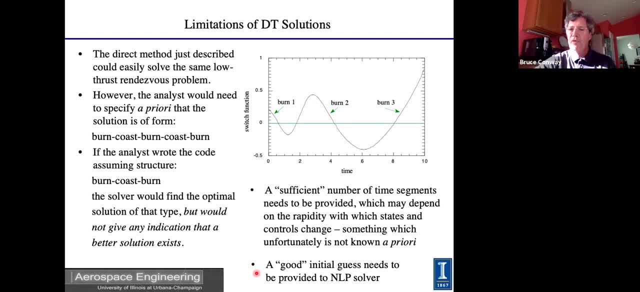 you need to give it a good initial guess in order for it to converge, And then you still have the same problem that the solution tends to be in the neighborhood of the initial guess that you give it. So you still have this problem of possibly converging to local minima when there's a better global minima. 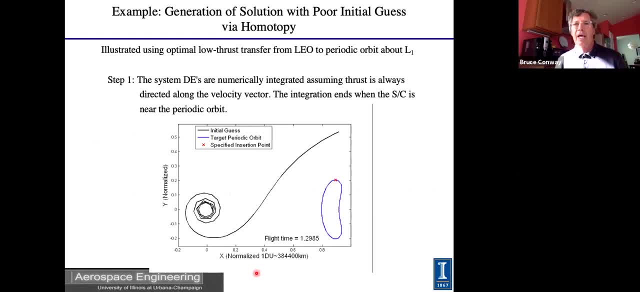 Let me just give you a simple example of a complicated problem where you really have no idea of what a good initial guess would be and how to get around it. So this is a problem that we solved on our way to solving a more complicated one. 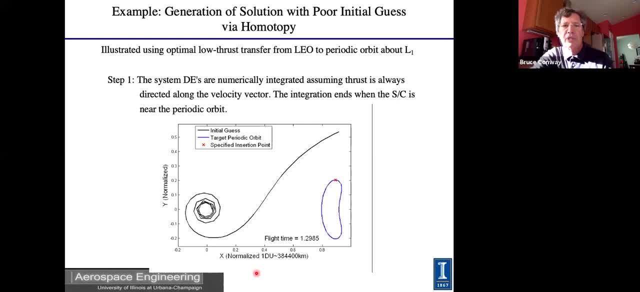 I'll show you a figure of that before. But let's suppose that we want to use low thrust to go from low earth orbit and enter and then remain in a Lyapunov orbit, which is a 2D halo orbit centered on the interior Lagrange point in the earth-moon system. 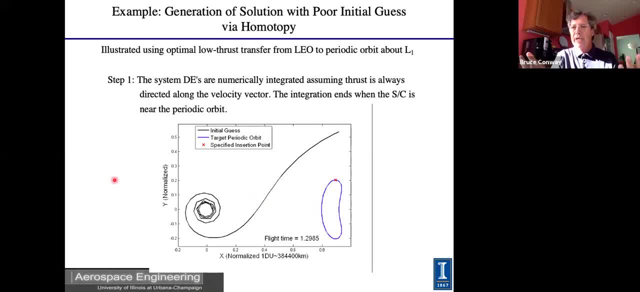 Okay, But we have no idea what a good initial guess for that trajectory is. It's quite complicated, you can see, because it has many revolutions around Earth before you get escape energy. So the first step, let's assume that the thrust is always directed along the velocity vector That maximizes the rate of increase of 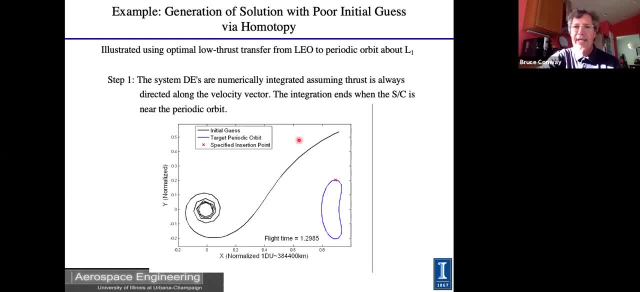 kinetic energy. Well, and then stop the integration when you get anywhere near the final orbit. Well, that gets you close, but it's not great. You do have to pick the right starting point, because if you don't, you'll end up going off to the left instead of off to the right. But that's trivial. 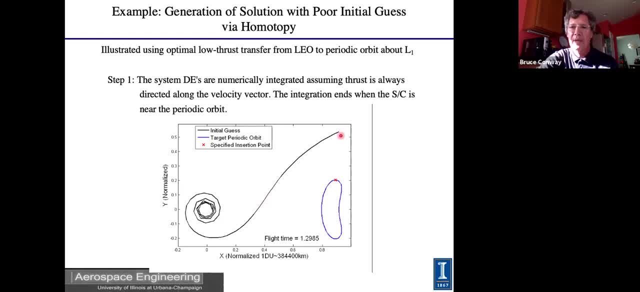 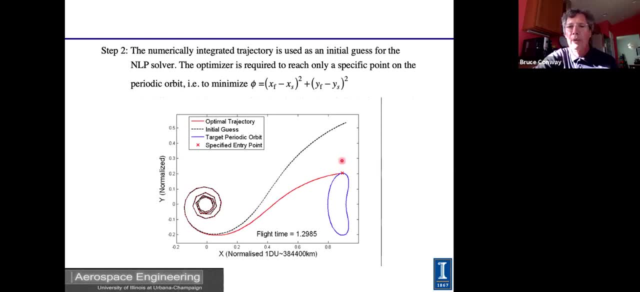 So we pick a good starting point, we get here. So then the next step is to use that as an initial guess for a second nonlinear program where we require to hit a specific point on the orbit, But still not necessarily the one that minimizes the fuel use. Then we take that red trajectory. 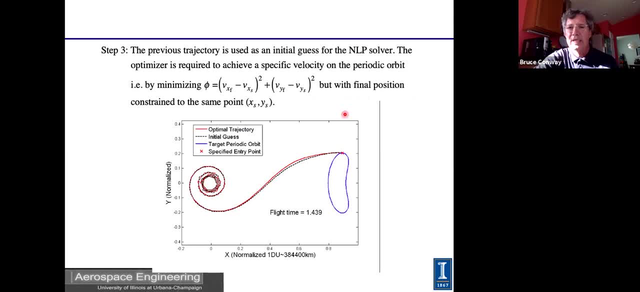 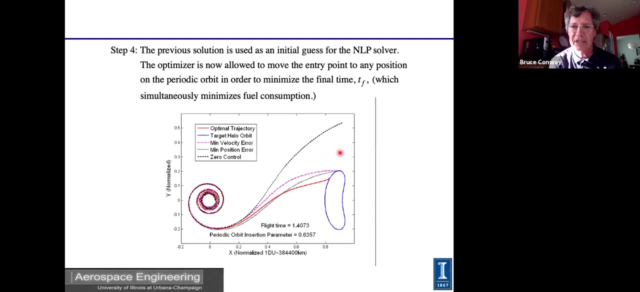 and we use it as an initial guess for a third solution that not only arrives at a point on that trajectory but has just the right velocity so that it would then follow that Lyapunov orbit. And then, finally, we use that as an initial guess for a fourth solution that relaxes the location constraint. 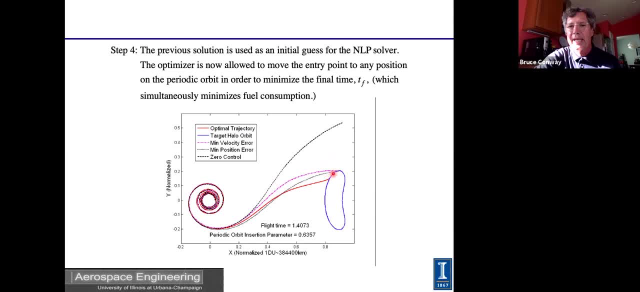 and says, okay, now find an entry point anywhere on that orbit if it minimizes the fuel used. So you see now how you can start with absolutely no idea what a good initial guess is, and with a homotopy you can still solve the problem, But it's it's a little time consuming. 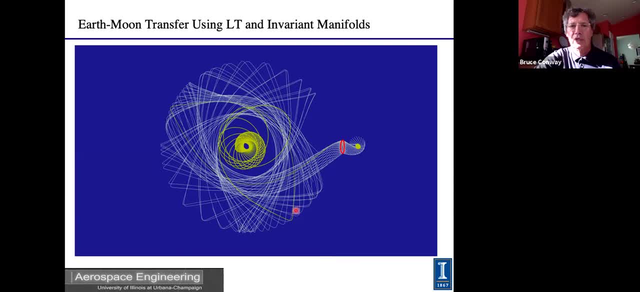 The real problem we wanted to solve was this one, which is a low thrust transfer from low Earth orbit to a low lunar orbit orbit Using invariant manifolds. you probably know about those. Those are coasting trajectories in the three-body problem. So we used a method very similar to the one I just showed you. 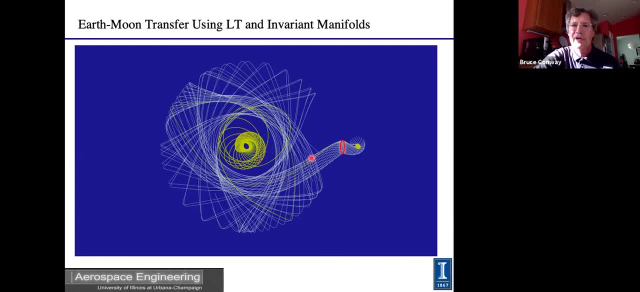 to find a trajectory that takes the vehicle and enters a halo orbit around the interior Lagrange point, then departs that orbit and goes to the moon. What looks like the moon there, this yellow thing, that's actually a very, very close-knit spiral that goes down to a low lunar orbit. 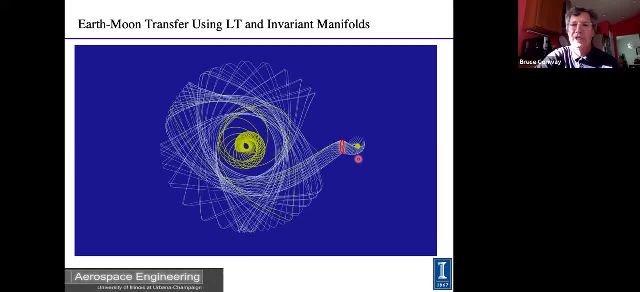 This is an extremely complicated problem. We actually used it as the cover art for the other book that Siegfried mentioned on optimizing space trajectories. So if you're patient enough, you can get these direct methods to solve very complicated problems. Okay, Well, in about the 19th. 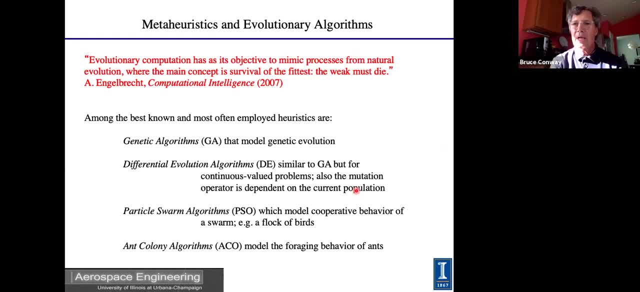 1990s, people realized that it would be really nice to come up with a solution that is not prejudiced, That is to say, that doesn't require an initial guess of the solution, And methods that are initialized totally randomly are evolutionary algorithms. one that you probably all know is a 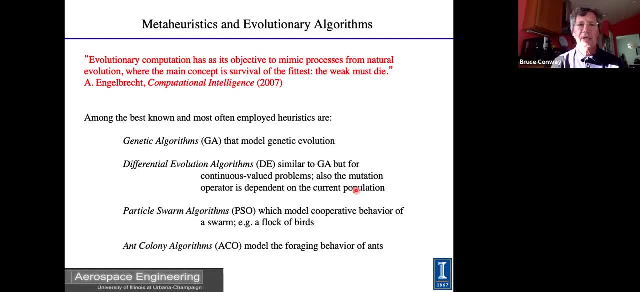 genetic algorithm or a heuristic like particle swarming. Okay, Well, in about the 19th 1990s people realized that it would be really nice to come up with a solution that is not prejudiced, That is to say that doesn't require an initial guess of the solution And methods that. 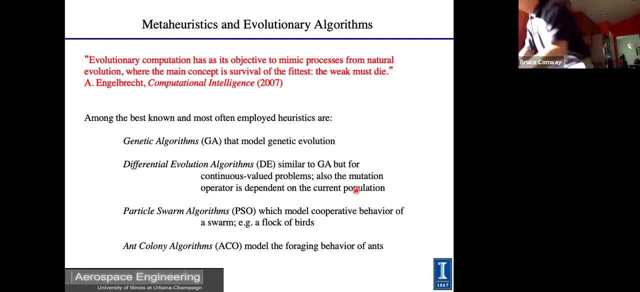 are initialized totally randomly are evolutionary algorithms or a heuristic like particle swarming Or ant colony algorithms- Let me get rid of this sunlight here. So these are really nice because they don't require any a priori information about the solution, So you don't prejudice it to look in a certain neighborhood when you use these methods. 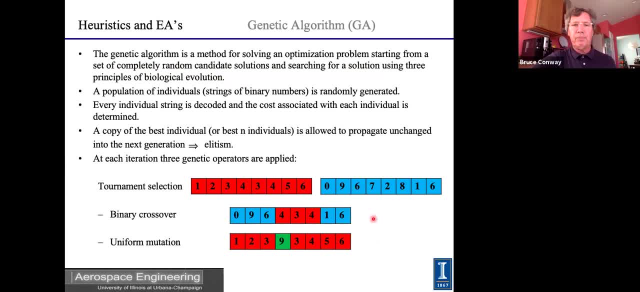 Let me just say just a little bit about genetic algorithms. algorithm if you're not familiar with it. the basic idea is to create chromosomes. that are strings of numbers. it can be binary. this one is is is not binary, but it's the same idea, suppose in this. 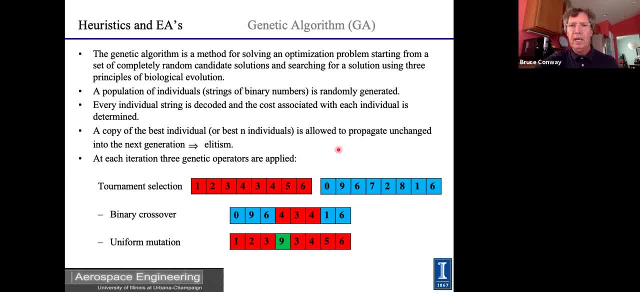 case, we have strings that are eight elements long and you create some large number of them- maybe 500 of them- and each one can be decoded to tell you something about the space mission, and it can be decoded and give you a cost. so, for example, the first three numbers here could be the, um, the 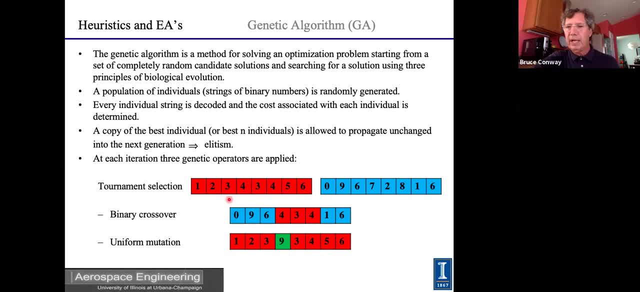 departure date, following some given epoch date. the next two could be, let's say, the uh, the time that the astronauts are, um, you are, on the surface of the object, asteroid, or maybe even mars. and then the third numbers could be the. these three numbers could represent the number of days after the uh, after the stay that. 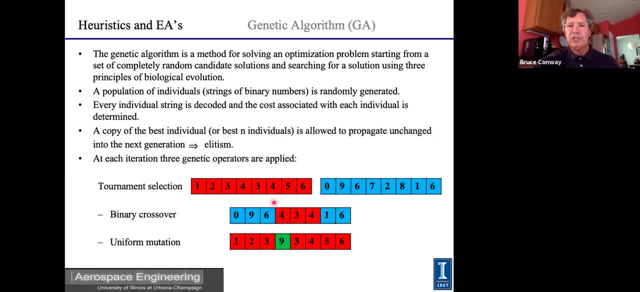 you arrive back on earth so that information is sufficient to solve the lambert's problems, to give you a delta v cost for the mission. so you generate, let's say, 500 of these strings randomly and then you evaluate the cost of every one. then let's say you throw away the worst 250. 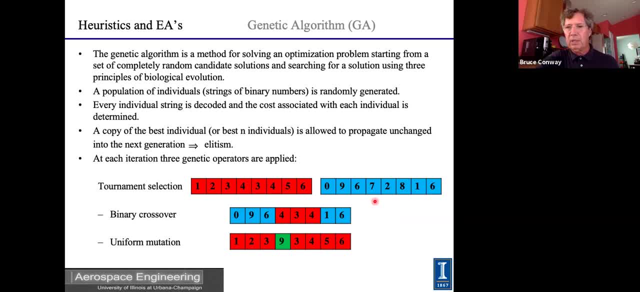 initially. a lot of them are going to be terrible. a lot of them may because they're random. they may have departure dates from the asteroid prior to the departure from the earth, so they make no sense. so you give them a ridiculously high cost, like a million, and then they'll remove themselves. 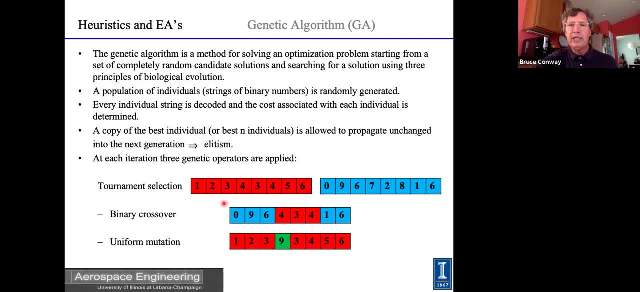 so you remove the high cost ones, you take the remaining ones and choose them at random to become parents for an offspring. you select pieces of the parents to create in a random way to create children, and then in a very small number, usually around half a percent, you just flip one digit. 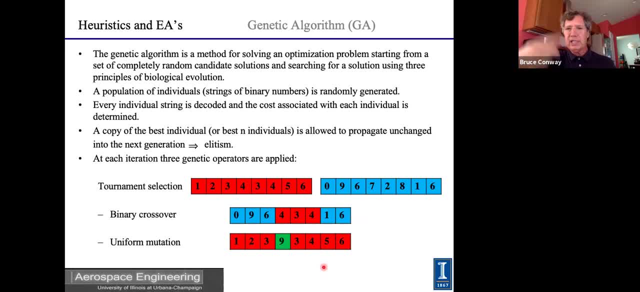 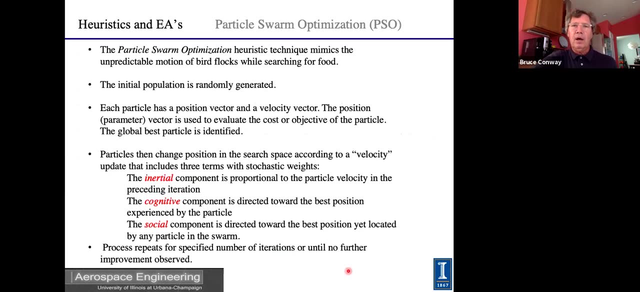 randomly and then the process repeats. and as the process iterates, the solutions generally get better and better. you can run it until you reach a certain goal, or you can just run it for an arbitrary number of generations. particle swarm is qualitatively different because it's not an evolutionary technique. in this case, 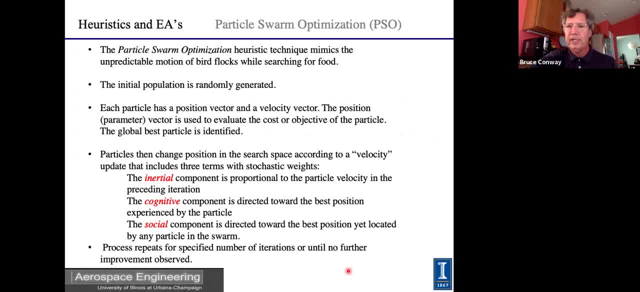 every individual particle is trying to improve his or her cost. they're trying to improve themselves, but the initial population is still randomly generated. so every particle is initially generated and then every particle is generated, inserted in an n-dimensional space. then the coordinates of the position are used to evaluate. 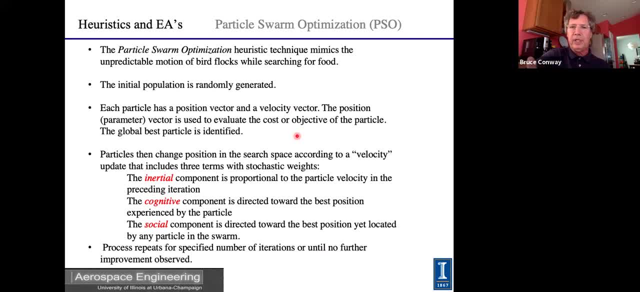 the cost. in exactly the same way that it was done with the genetic algorithm. It's decoded and a cost is arrived at, A global best particle is identified and then in the next step, or in each successive step, the particles move in this n-dimensional search space, They take a step. 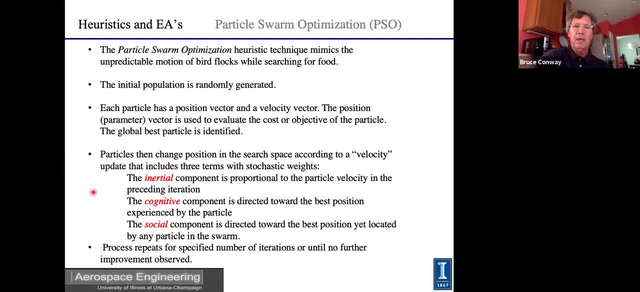 it's referred to as the velocity, but it's really a displacement. They move with a vector that's the sum of three. it's a linear combination of three vectors. The first is the so-called inertial component, which means take a step in the direction that you were moving at the last step. 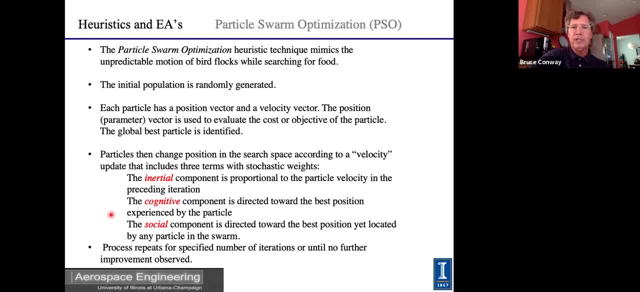 The second step is called the cognery. The cognery is a cognitive component which says: move towards the best position that you personally have ever experienced. Now, that's in there, because it's possible in this method for a particle to move away from or to move to a new position that's worse than the position that it 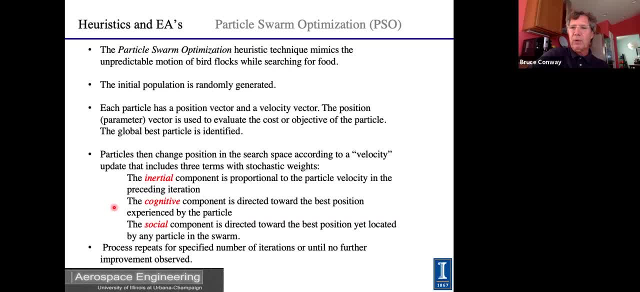 was in. So this one's saying: take me back to where I was, because it was better. And then the third one, which is the most important, is the social component, which says: take me towards the particle that has found the global best location. Now, each of these three vector, 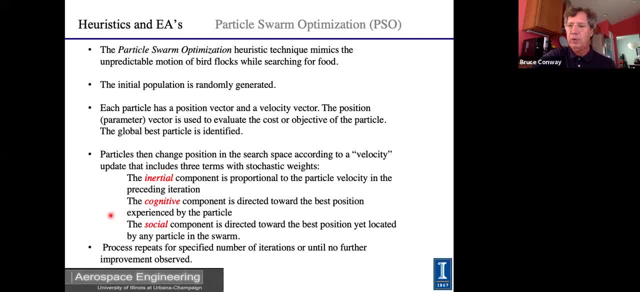 components is multiplied by a random number between zero and one. So it's quite stochastic. because the initial population is randomly generated and because each of these components is multiplied by a random number, you can run the PSO and you never, of course, get the same. 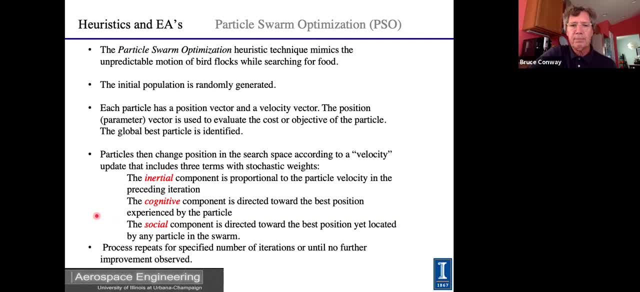 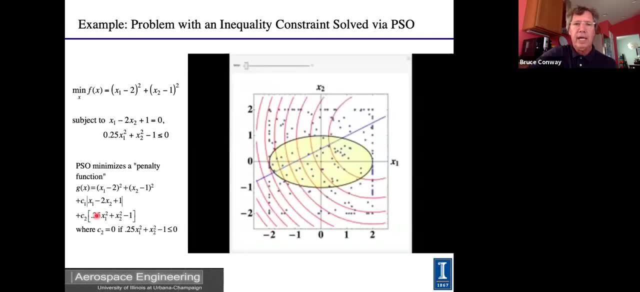 result twice, And then you repeat the process for a fixed number of iterations or until you don't see any more improvement. Here's a simple example: Shoot Well for some reason. Well, I've lost the animation. The object here is to minimize a simple function of two parameters subject to constraints. Now I 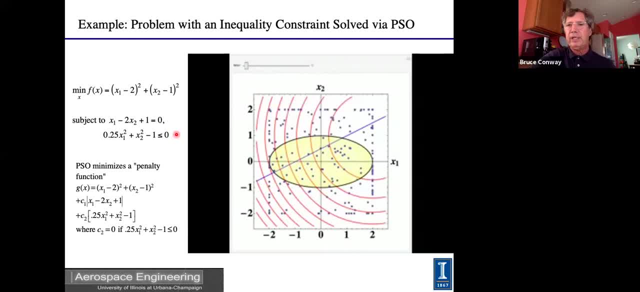 didn't really say much about that. So in today's model, in this model, there's no workout constraints. There's no native way to handle constraints in these heuristic and evolutionary methods, except to add them as penalty parameters. So you add the constraints to the function you want to minimize and through weights, here called 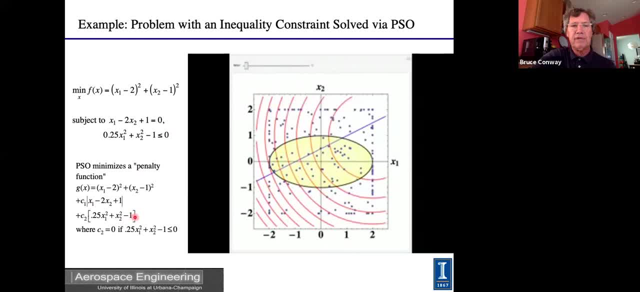 C1 and C2.. And then the optimizer can minimize it if it drives the constraints to zero. So in this case we're trying to minimize this function, the particle, uh, that the solution lie on this straight line and that it'd be on the interior. 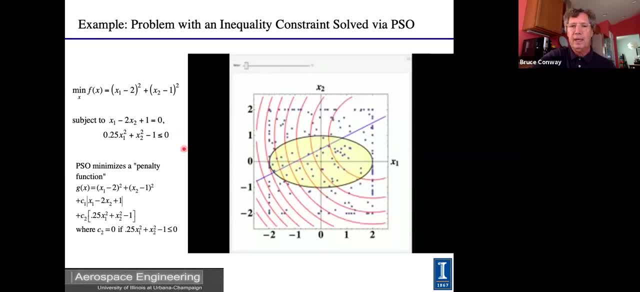 of the ellipse that's given by this equation and, unfortunately, up to now it was working, but it no longer. maybe it's because, yeah, maybe it's because it doesn't realize it's uh, turn that off, let me. ah, here we go. it didn't like it being a laser pointer, okay, so here are the particles moving. 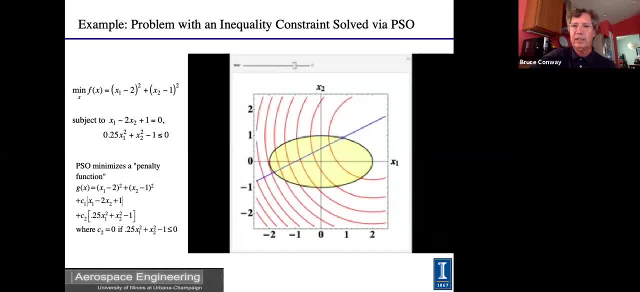 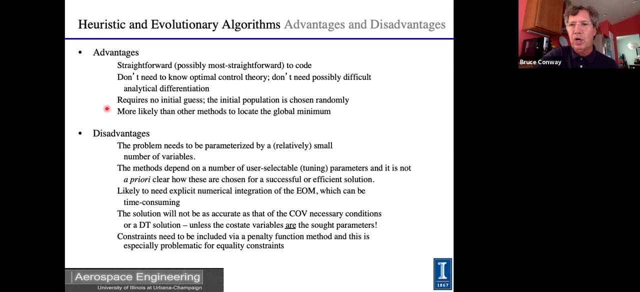 in a two-dimensional space and you see that they very quickly converge on the optimal point. okay, well, i'm really just going to talk about the advantages. it's really easy to code. i'm extremely easy to code. you don't need to know anything about optimal control theory. you don't. 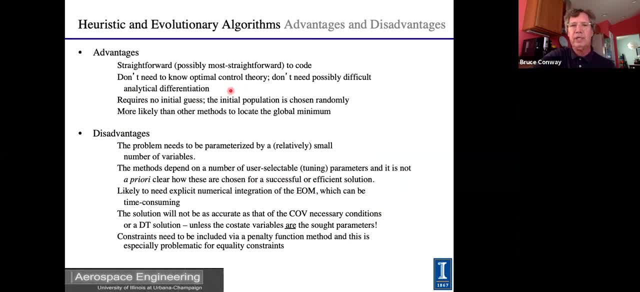 need to to know about Euler-Lagrange equations. A high school kid could do this, But the most important thing is that you don't have to prejudice it with any kind of initial guess. Also, if you use a large enough search space and a large number of particles, you're more likely than the other. 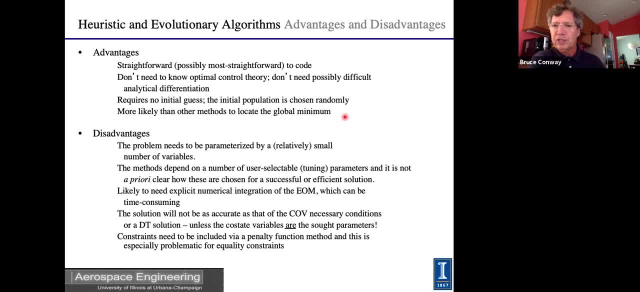 methods to find the global minimum, because they do a very efficient search of the space. And if it doesn't find it on the first try, you never are satisfied with doing it once. You run this thing multiple times and then you can be fairly confident that you found the global minimum. 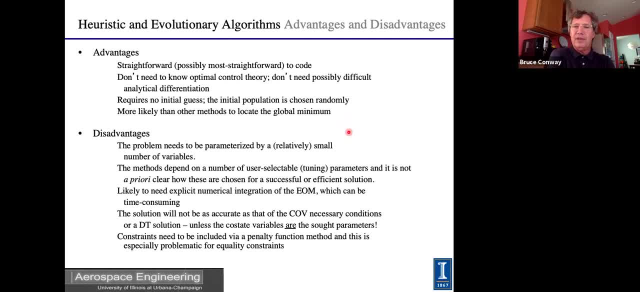 In fact it's funny If you watch these things iterate their animations on the web. it looks like a swarm of birds going after some kind of prey. You'll see the particles all head for a point which turns out to be a local minimum, And then one of the particles 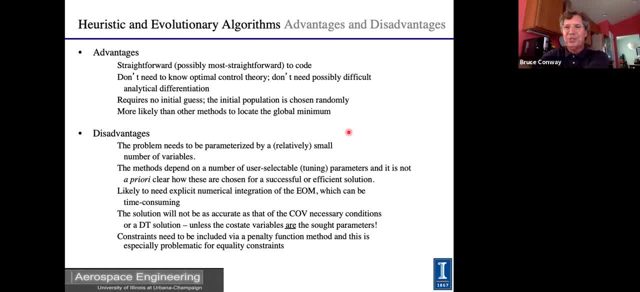 will find a lower cost, And then the entire swarm will turn and head towards that point. It's quite fun to watch. Of course, once you get above three dimensions, you can't watch it anymore, So here's a simple example. The one main disadvantage is that you have to parameterize. 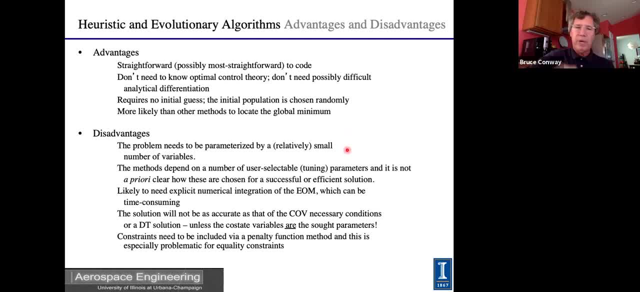 it with a small number of parameters. I mentioned that for the direct transcription solutions you can have thousands. We've solved problems with 3,000, 4,000 parameters. Here you have to use typically less than 100. So you have to find. 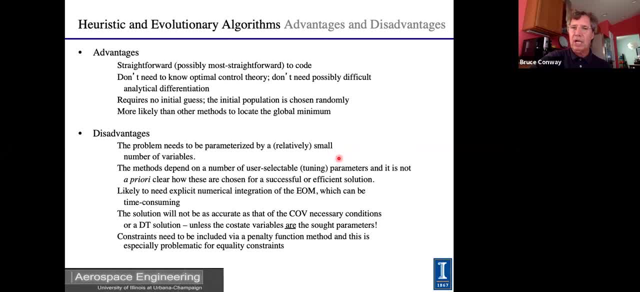 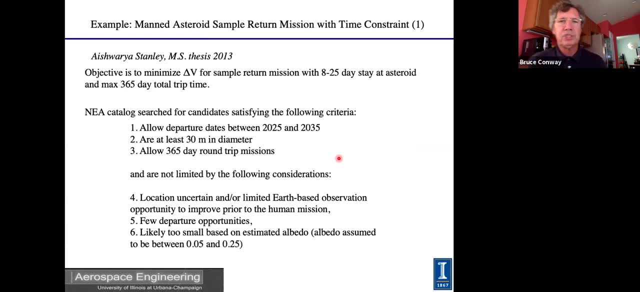 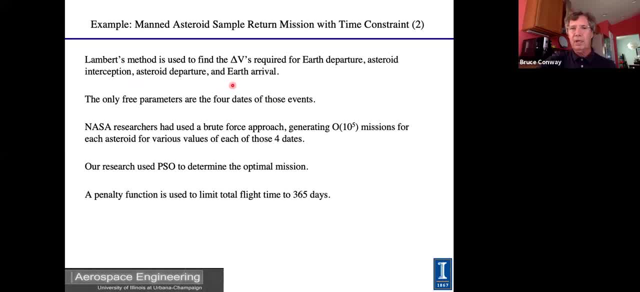 and the earth arrival. so there are only four parameters. but if you have a wide range of values for those, you you have to do um on the order of 10 to the fifth missions. it's a brute force approach. we decided to do it with p, with the particle swarm. 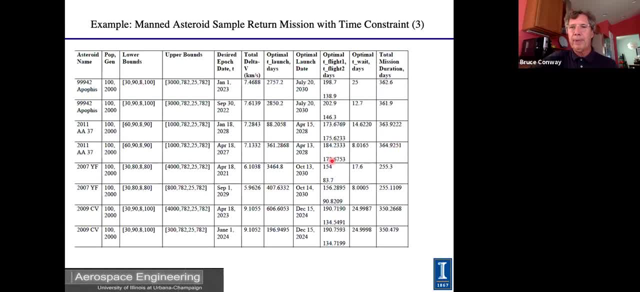 and here is just one page from her. she had like 10 pages of results. i won't go through a lot of them, but just to give you an idea, you probably all are all familiar with apophis, which is not just a near-earth asteroid but a potentially hazardous one. 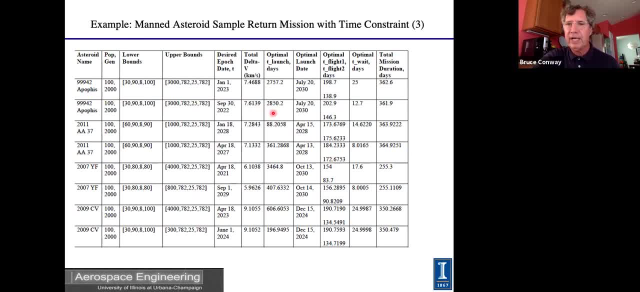 but this shows two different possible flights found by the particle swarm and this is done in hours on a laptop. for all of them together, it finds an optimal launch date, it finds an optimal time for the outbound flight, an optimal stay time at the asteroid and then um the total mission. 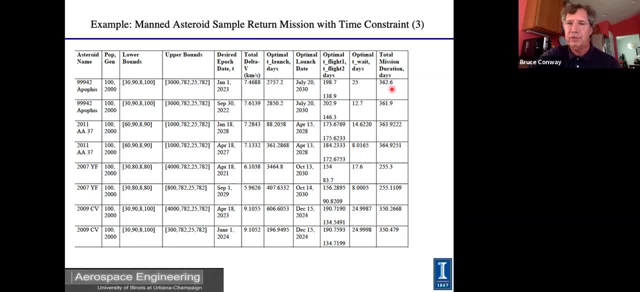 duration, so which effectively gives you the return trip time, and we did this for quite a few asteroids and it found very good solutions, much easier than what the people at nasa had done with a brute force approach. notice that some of them bump up right against the limits. the upper limit for the stay was 25 days. 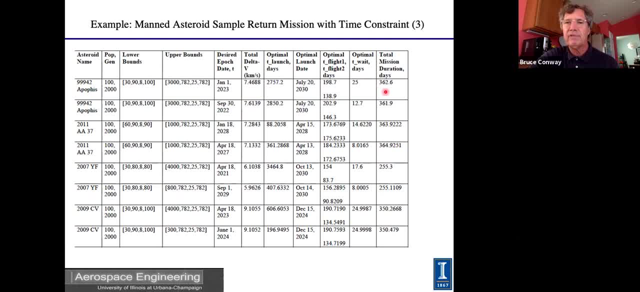 the upper limit for the mission duration was 365 days, but not all of them. here's one that's not close to either upper limit. when you're an optimization person, you see the upper limits being bumped up against the upper limits and you see the upper limits being bumped up against the. 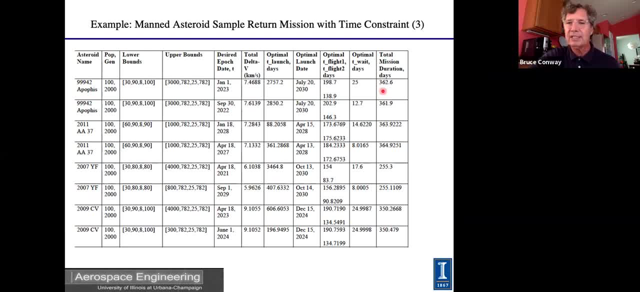 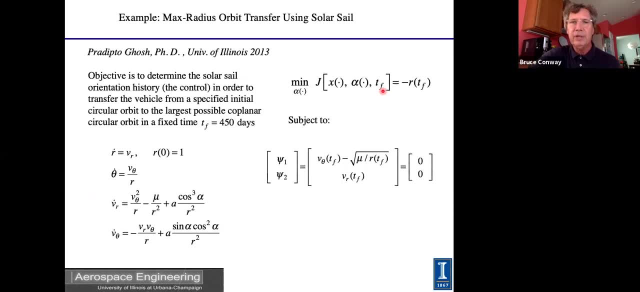 upper limits and you see the upper limits being bumped up against like this. what it's telling you is that if you can relax them, you do even better. but we, we took the same numbers that the nasa people used. here's another example. i won't go into a lot of the detail. it's a maximum radius orbit transfer. 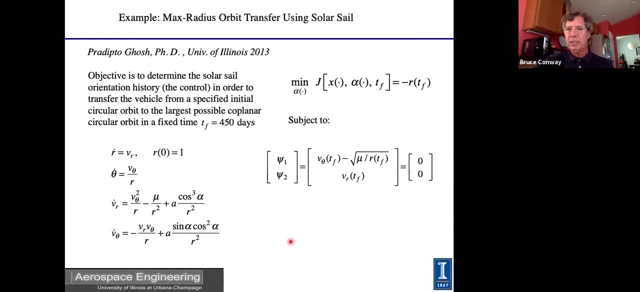 for a solar sail. so this is continuous propulsion, but not electric, and the idea was to find the solar sail orientation angle, this angle alpha in the differential equations that allowed a transfer from one au, a circular orbit at one au, to the largest possible circular orbit in a fixed time of 450 days. and the way he cleverly parametrized this was to describe that. 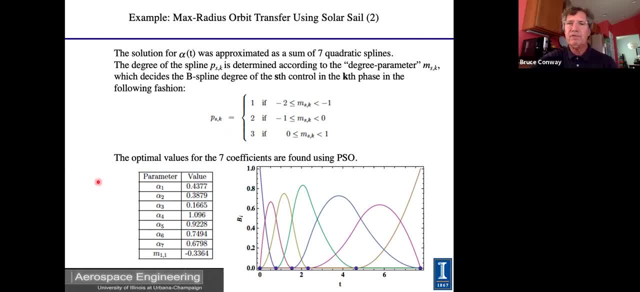 time history alpha as a sum of seven quadratic splines with coefficients given by these quantities, alpha one through alpha seven and the pso found the optimal value of the time history alpha is equal to zero. so this is the dynamic equation job and spline division. it had to put that all together. 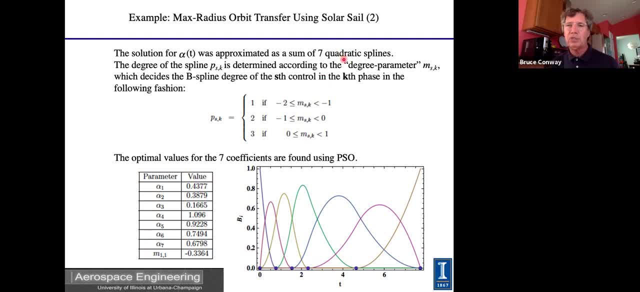 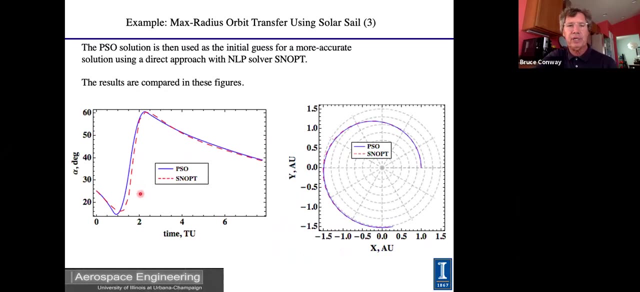 into one double division up and down versus his limit. so the jab Labor explained the cardiac linear десятiles plus the parametrous stop and down discriminant of the solar sail and the electromagnetic standard vector, math. and then they gave greenid in blue, like this as an uh: 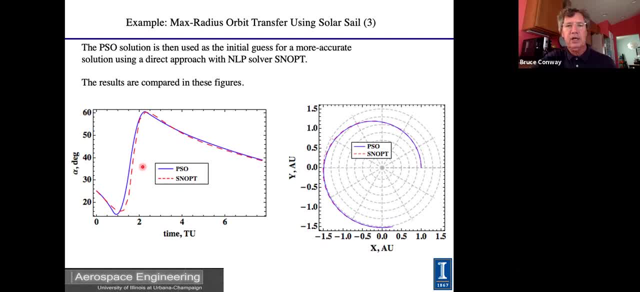 given by the idea of quantum prediction effect. and when you write permutation in grayscale, let's say for a direct transcription method, as I've described earlier, And that's the dotted line, You can see that they're almost on top of each other. It did a really, really good job of finding. 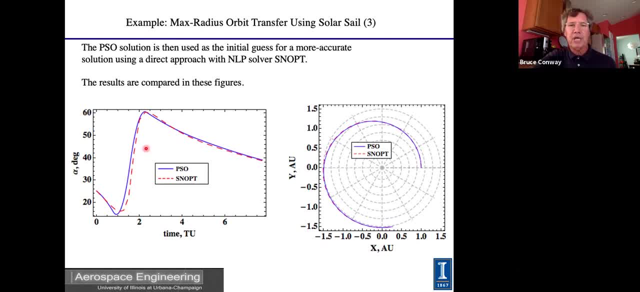 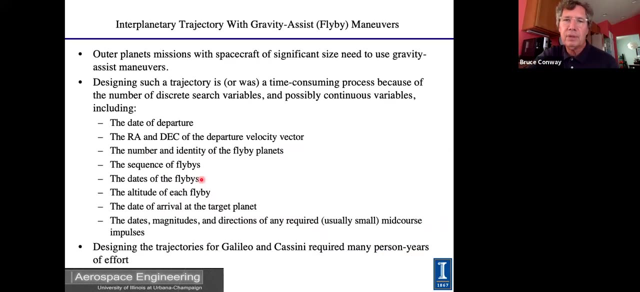 a solution. So it used just a handful of parameters, about eight, whereas the direct transcription solution needed thousands, And this is also faster. Okay, So now let me conclude with the most challenging problem for mission planners: The interplanetary trajectory with gravity assist maneuvers. This is the Galileo or Cassini trajectory problem. This is a difficult problem Even if you use- assume importance- pulse of chemical thrust, which is what they use, not low thrust. It's difficult because there are so many free parameters: The date of departure, the RA and declination of the departure velocity vector, which planets to use for flybys. 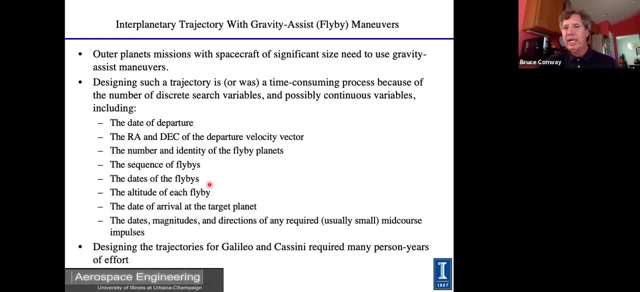 and in what sequence? what will be the dates of the flybys, what will be the altitude of each flyby and the date of departure? What will be the optimal date of arrival at the target planet? And then the dates, the magnitudes and the directions of any- I say usually small, mid-course impulses. 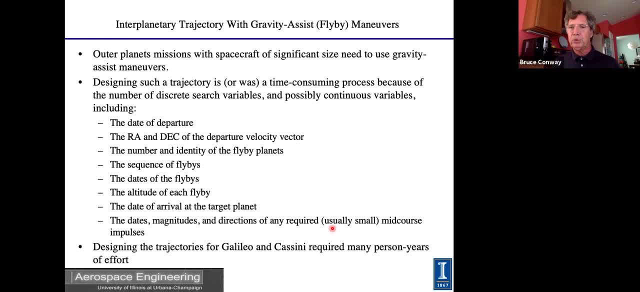 I say usually small, because at this point in the trajectory the vehicle is no longer connected to an upper stage of the launch vehicle, So any fuel it uses is fuel that it can't use for extending its lifetime at Jupiter, for example. So you really have to think about the trajectory. You really want to minimize that. It'd be nice to have a trajectory that doesn't need any mid-course impulses, but sometimes small ones are required just to help set up the one flyby for the next flyby. Designing trajectories for Galileo and Cassini was a many-person year effort. I know a lot of. 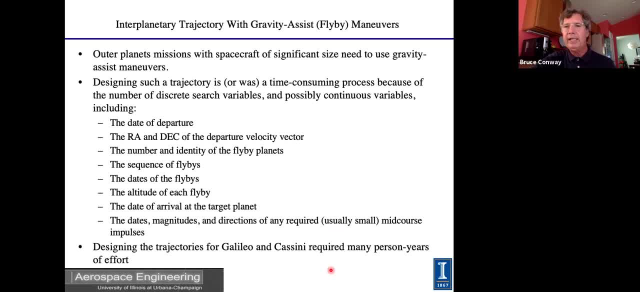 the people who worked on it- and it was a big problem- aided, of course, by their experiences orbital mechanicians, They were able to rule out a lot of problems. They were able to rule out a lot of possibilities, because they just don't make any sense. 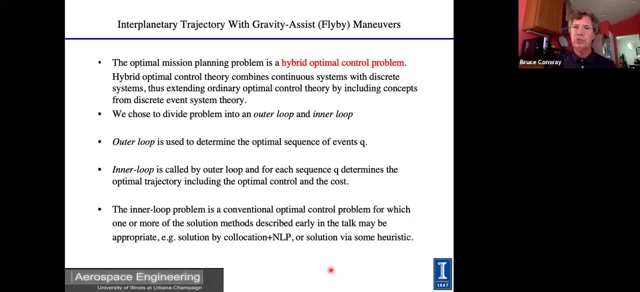 This is referred to in control theory as a hybrid optimal control problem. That is to say, there are a number of discrete parameters that the solution depends on, and then there are continuous parameters like the radius, the azimuthal angle- in the earlier terms, the r, the theta, the v sub r, the v sub theta, and so on. 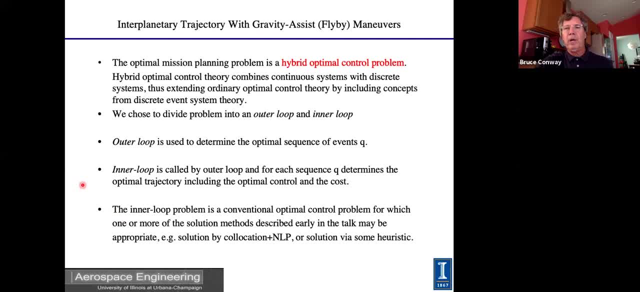 The way we chose to solve the problem is really pretty much the only way you can approach these hybrid optimal control problems, which is to divide the problem into an outer loop and an inner loop. In our case, we use the outer loop to define the identities and the sequence of the 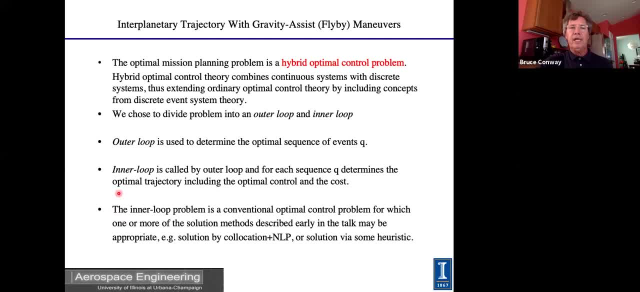 planets to be used for the flybys. The inner loop is then called by the outer loop and it says: okay, you're going to use these planets in this sequence, assuming that What is the optimal trajectory? Find me all those other things, the dates of departure. 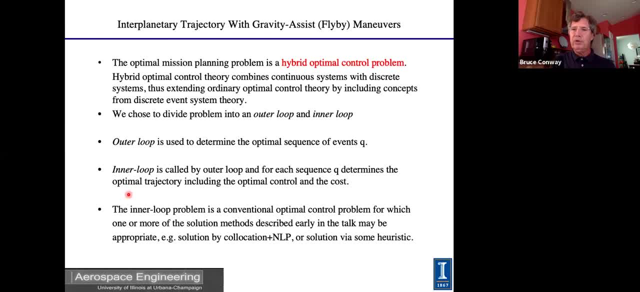 the date of each flyby, the altitude of each flyby, et cetera, in order to satisfy the mission constraints that you've given me. Then the inner loop returns the cost of that trajectory, if it's at all feasible, back to the outer loop. So that inner loop problem. 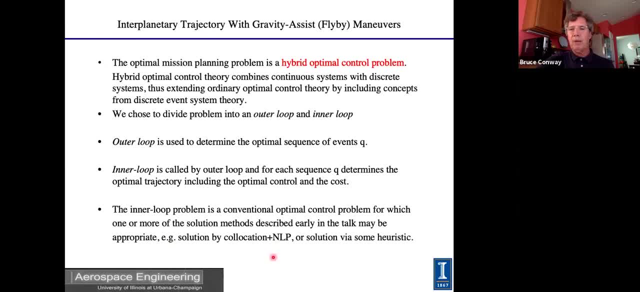 as I said, is a conventional optimal control problem. You can solve it with the methods that I've described. You could set it up as a Transcribe it into a nonlinear programming problem or, in this case, we actually used another heuristic that I didn't describe. It's. 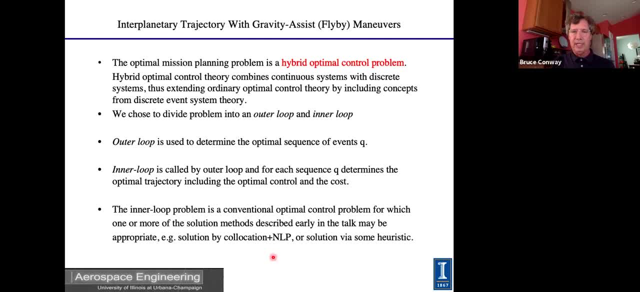 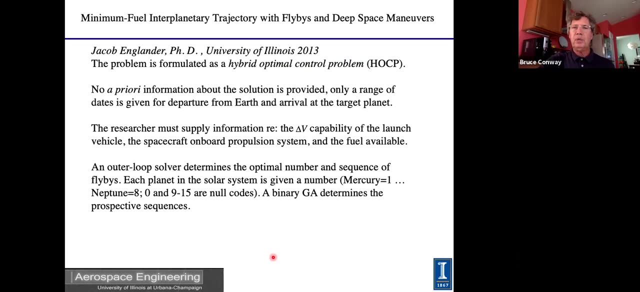 too messy to describe in detail here, called differential evolution, But it's just another evolutionary algorithm. So one of my PhD students then tried to automate this mission planning process, basically to automate what was done by the people at JPL for Galileo and Cassini. 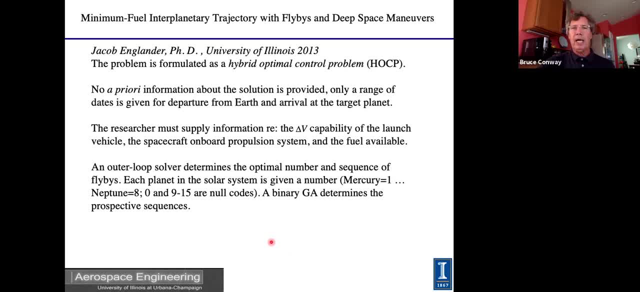 And he actually relied on work of two previous PhD students. It was really an effort that took place in the early 2000s And he was able to do it. And he was able to do it in the early 2000s. 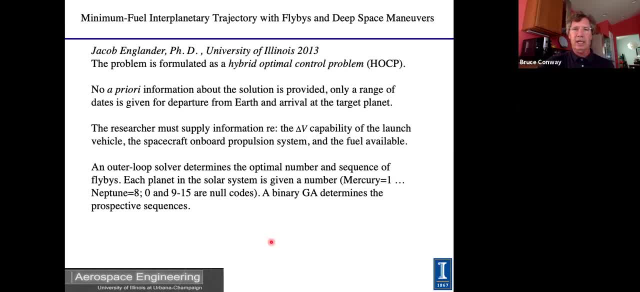 Over a decade, they had each made advances that allowed Jacob to actually complete the goal. So we wanted to create an automaton that would solve this complicated mission planning problem, with almost no a priori information provided, Simply a range of dates that are allowable. 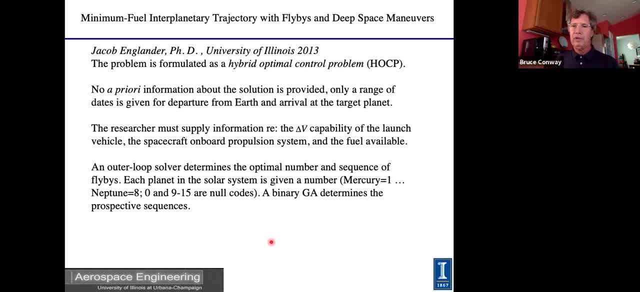 for departure from Earth and allowable for arrival at the target planet. Then, of course, you do have to give it information about what launch vehicle is being used, so that you know what your velocity- hyperbolic excess velocity- will be when you leave the Earth. You need to provide a little bit of information about the onboard propulsion, so you 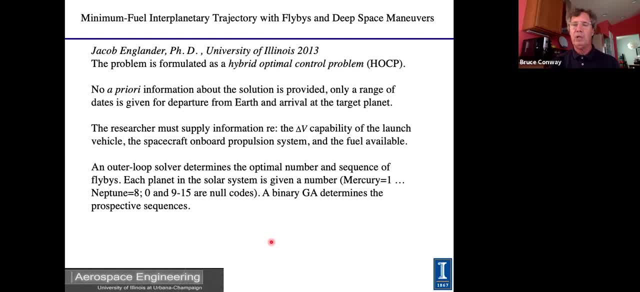 know how much fuel would be consumed in a mid-course impulse, Just basic stuff like that. But no, you don't have to supply any information, any instinct as to what the solution is going to be, And then you can give it information about how the aircraft will function as well. 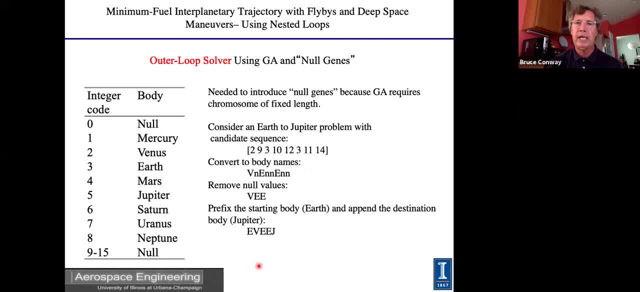 So that's one of the things that we're going to be looking at. The second part is going to be more about the technology and how the propulsion will look like. With regard to the outer loop solver, we used a genetic algorithm, And the easiest thing with the genetic algorithm is to use a base two number for the length of the chromosome. So either four, eight or 16 parameters or numbers. We needed to use 16,, but there are only eight possible planets that we could use for full-time, So that's a pretty big deal. And then we needed to use a base two number for the length of the chromosome. 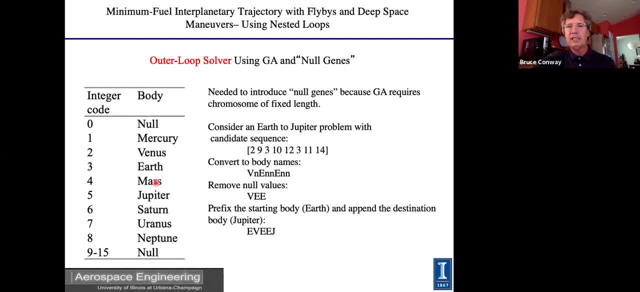 And then we needed to use a base two number for the length of the chromosome flybys. so the student came up with this concept of using null genes, meaning that a ga string like this: 2, 9, 3, 10, 12, 3, 11, 14, would decode to venus, which is body 2. the 9 is a null code, there's no. 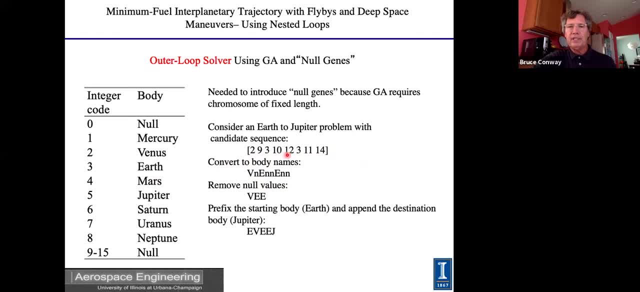 planet, then 3 is earth, then 10 and 12 don't correspond to any real planets. 3 is earth again, and 11, 14 are both non-existent planets. so when you decode it you get venus, earth, earth and some null planets. you remove those and you prefix the starting body, append the destination. 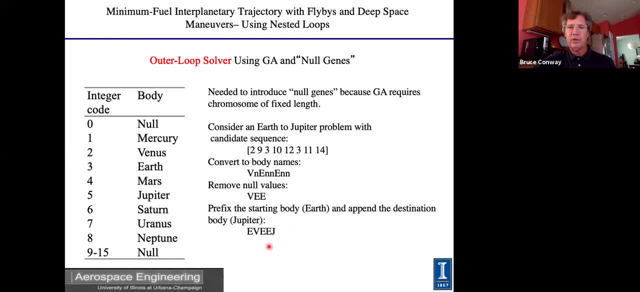 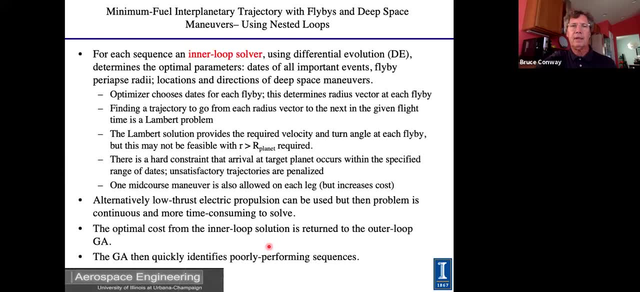 body. and there's your sequence: earth, venus, earth, earth or depart. earth, venus flyby, earth flyby, another earth flyby, arrive at jupiter. then the inner loop, solver, i, i. i. I'm kind of running out of time here so I won't go into a lot of description about it, but 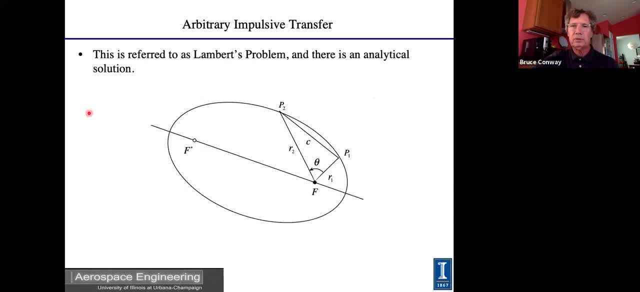 I described a Lambert problem which looks like this. so if the date for a flyby is known, you know where the position of the flyby planet is. if the date for the next flyby is known, you know where that planet will be. you then know this interior angle and the lengths of those radius. 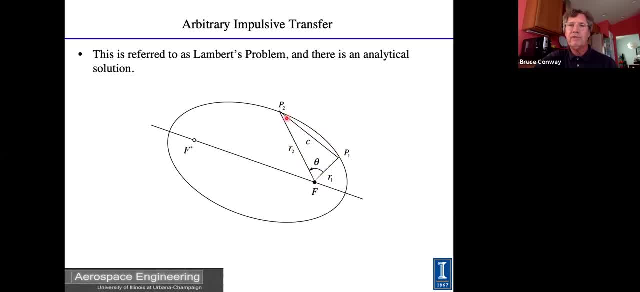 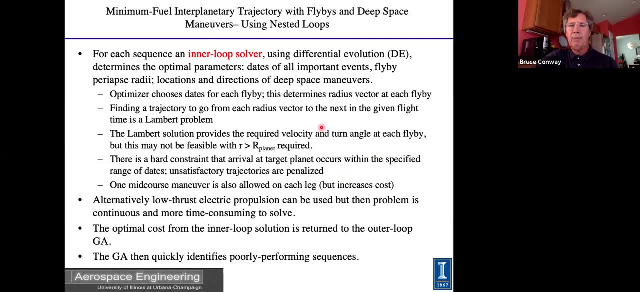 vectors and you know the transfer time so you can find the elliptic arc that connects them. so the individual problems going from one planet to the next are Lambert problems. they're relatively easy to solve. the only complication is that the required velocity change from the flyby. 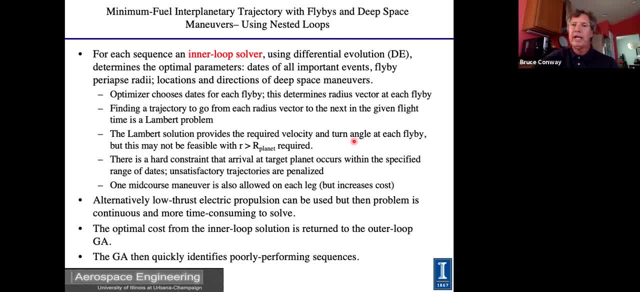 and the turn angle to set you off in the right direction. to go to the next flyby planet might require a flyby that's below the planet's surface, which isn't going to work, so it's very stupid to developivering it. so it's not the future for this. 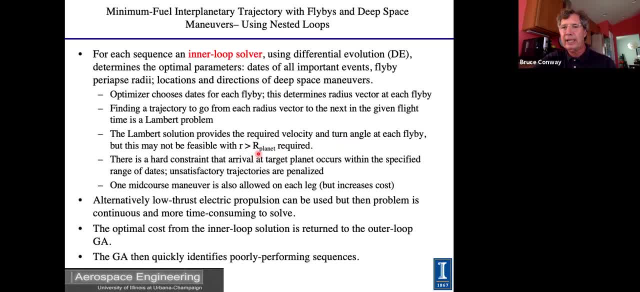 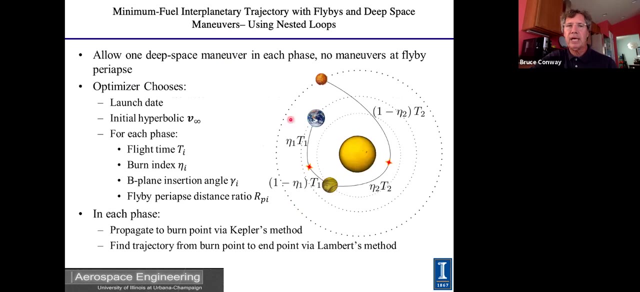 so we have to put in a requirement that the flyby altitude be above the surface of the planet. if you're going to have a licensure on the riser, you essentially want the секων, that it's ISA and a diatomite type of Lloyd麯. 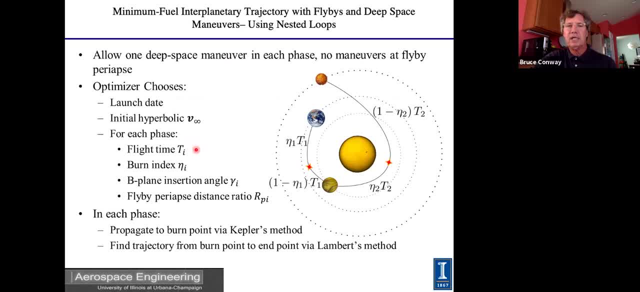 ск date, and then, for each phase, the flight time, which gives the arrival date at the next planet, and so on. A so-called burn index, which is a number between zero and one that tells you how much of the leg is used before you do the mid-course impulse. Most of the time, the mid-course impulses 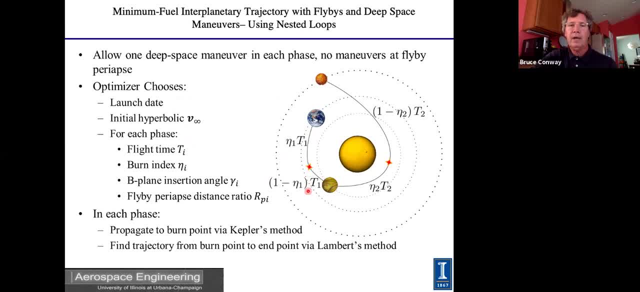 turn out to be zero or negligibly small. The so-called B-plane insertion angle at the arrival planet- I don't have time to go into detail about that- and the fly-by periaps distance rate ratio, which has to be bigger than one, otherwise you tunnel into the planet. 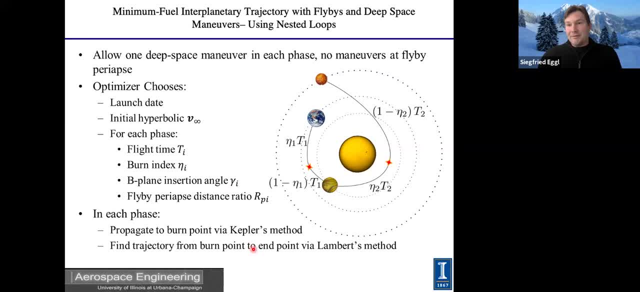 So sorry to interrupt you, Bruce, with just one second, So we are on top of the hour. so thanks everybody who has to jump ship, Thanks for attending and for everybody who can stay around a little longer. I'm happy. I think Bruce is happy too. 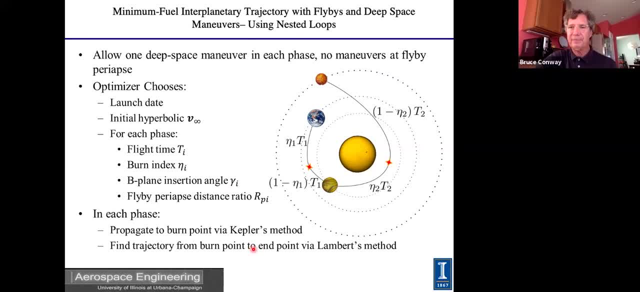 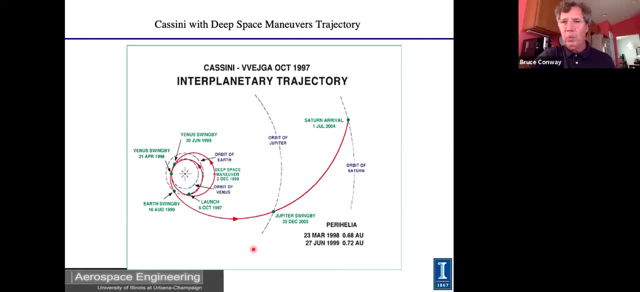 I have some questions. It's getting very close to the end, Thank you. So here's the actual trajectory for Cassini. Once we had this automaton written, we wanted to test it against an existing solution and we knew that this Cassini trajectory had been tested multiple times. The JPL people did. 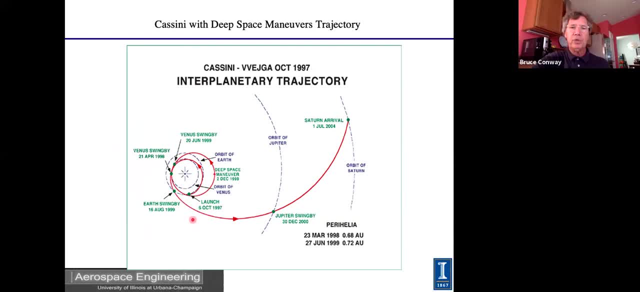 indeed find the best solution, And so you can see here's launch in October 1997.. Then there is a first Venus swing-by in April of 98. Then it goes around. there's a one mid-course maneuver in December of 1998.. Then it comes around again. there's a Venus swing-by in August of 99.. 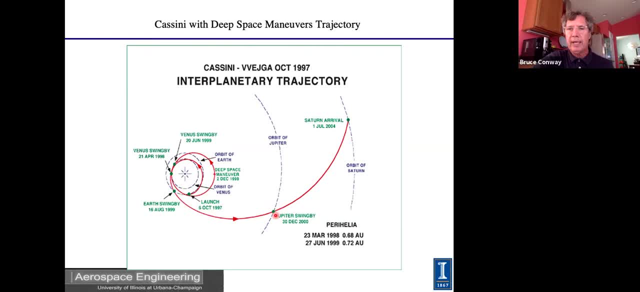 And then the spacecraft is on its way to a Jupiter swing-by, And then that took it to Saturn. So we were hoping to see if our audience was going to be able to see this, And it is. We were hoping for our own 500 years of work in the这么-time could be produced this with, as I said, 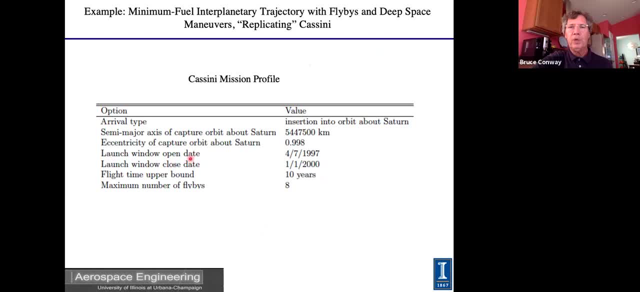 almost no a priori information. So here is what we told it. We told it the desired capture orbit radius, The desired capture orbit eccentricity, which all corresponded to the actual parameters, A launch window: open date in April of 97.. 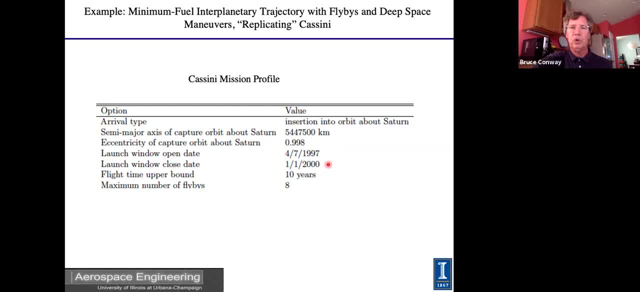 A close date in January of 98. of 2000, so a little more than two years open window, upper bound, a flight time of 10 years and then a maximum of eight possible flybys. of course we knew the answer was that there were only. 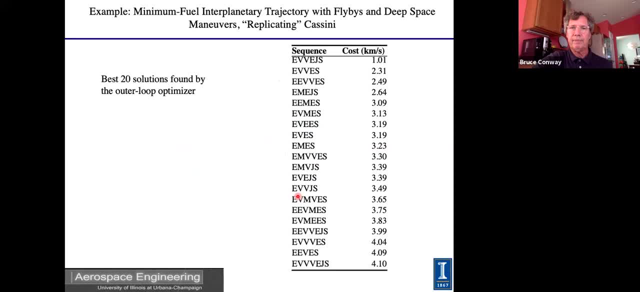 three, but we didn't use that, and here is what the optimizer came up with. it finds the optimal solution- venus, venus, earth, jupiter flybys- with a cost of just a little over one kilometer per second. these are the next 20 best solutions that the optimizer came up with. 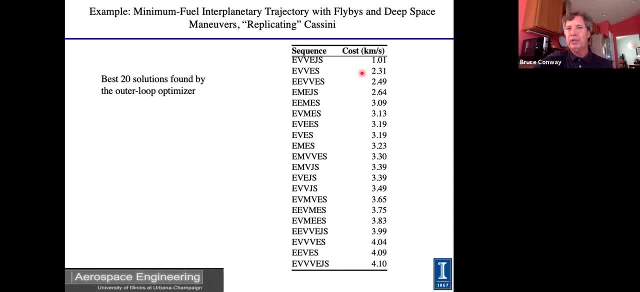 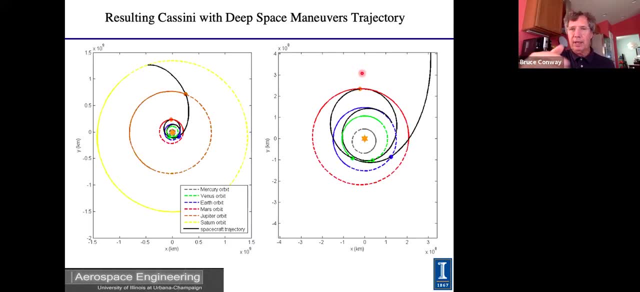 all of them are pretty bad, even that the, the next best one, uses more than twice as much fuel. here's what the uh. this is our solution, but it really is the best solution that the optimizer came up with. it really is the same one that you saw in the jpl cartoon, except this one's harder to visualize. 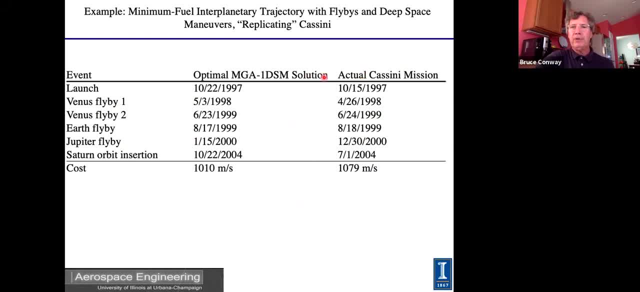 here's our result compared to the. this is our automaton solution versus the actual cassini mission. the launch date that our optimizer comes up with is within a week of the actual. the first venus flyby is also within about a week of the actual. the second venus flyby is just one day different. 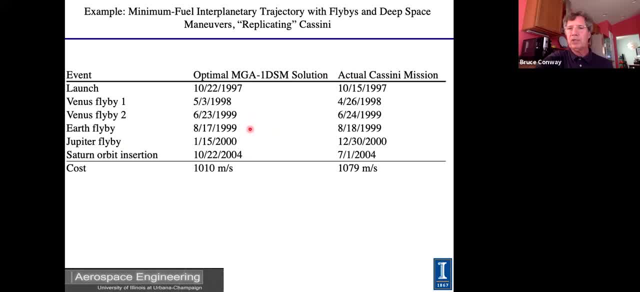 from the actual. the earth flyby is also just one day different from the actual. the jupiter flyby, however, is almost two weeks different and the saturn orbit insertion is substantially different. there's a reason for this. it's not the fault of our optimizer. the actual cassini mission had a sub optimal requirement. 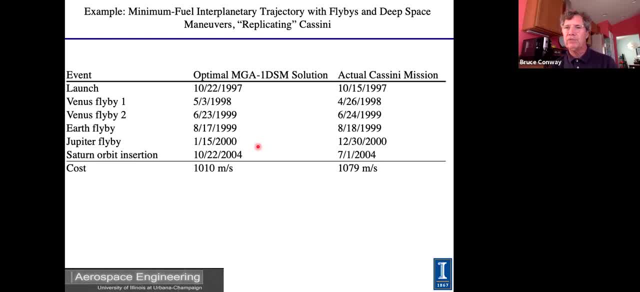 that when it arrived at saturn it did a close fly by of one of the moons- i think it was was Titan- which was not necessary to minimizing the propellant use, but it had a scientific purpose, But we didn't include that in our analysis. So up to that point of the Jupiter. 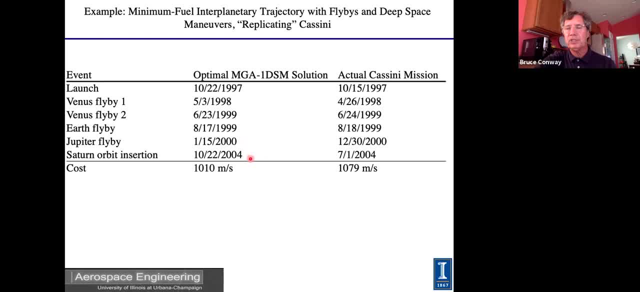 flyby, things are pretty close. And then the Saturn orbit insertion is different. because we didn't include that constraint, Our solution has a slightly better cost because, again, if you add some extraneous requirement like needing to fly by, do a close flyby of one of. 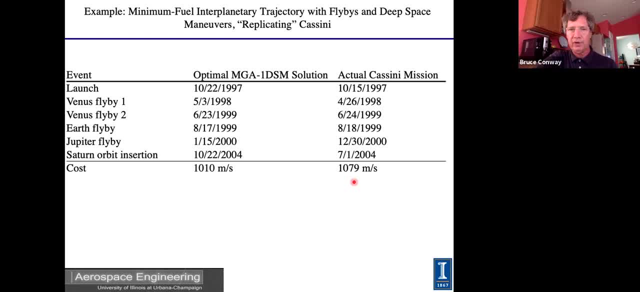 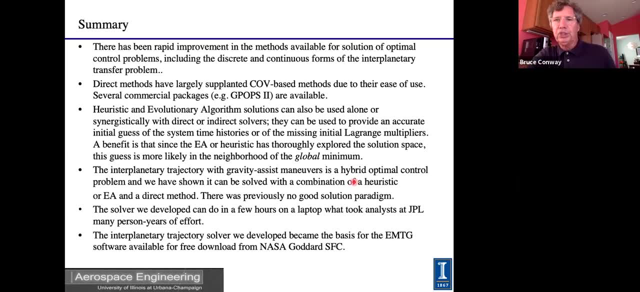 the moons as you're inbound. that's going to make the cost higher than if your only objective is to minimize fuel. So, in summary, just in my career, there's been a dramatic improvement in the methods that are available for solving optimal trajectory problems of any type. 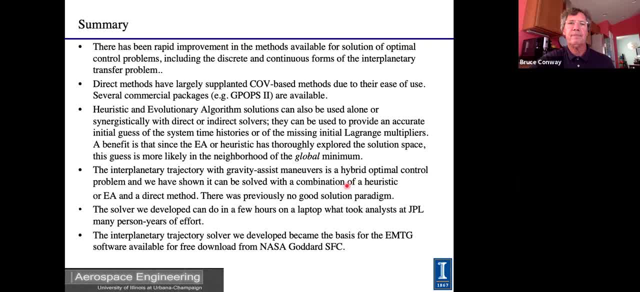 not just interplanetary transfers. The direct methods are generally much better to the calculus of variations-based methods, because they're just more robust than solving a two-point boundary value problem. Since about 1990, we've now found that heuristic algorithms and evolutionary algorithms 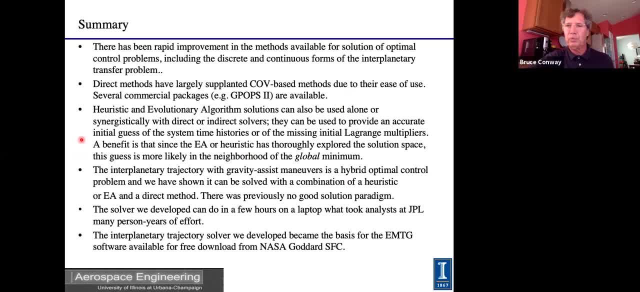 either can be used alone, if you're clever enough to reduce the number of parameters to a pretty small number, or you can use them, as you saw in this last example, to solve a two-point boundary example, synergistically with the direct transcription methods, And the advantage of that is that 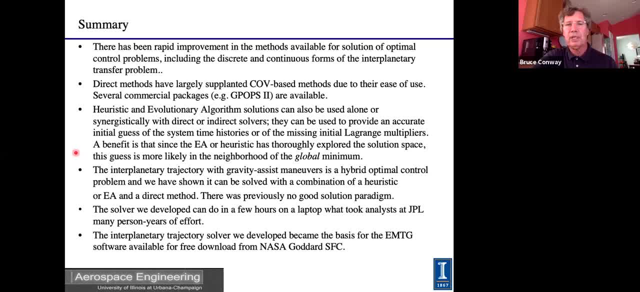 the synergistic combination allows the evolutionary algorithm or the heuristic to do a better exploration of the solution space and it's not prejudiced by any kind of initial guess. So I think that's it, Thank you very much. Thank you. So, as I said, what I described this automaton we came up with. what I didn't mention is that it works in just a few hours on a laptop and it replaces many person years of effort that were required at JPL to do Cassini and Galileo before that. 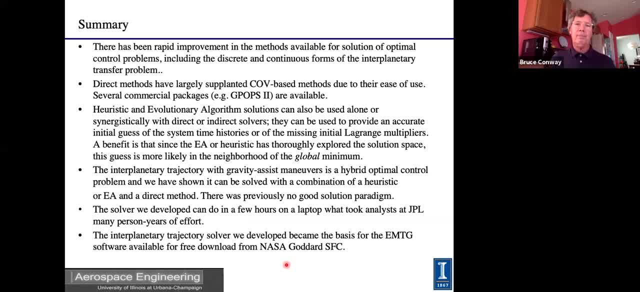 And, if anyone has any interest, this solver: NASA was clever enough to give this PhD student a uh scholarship. uh, forgotten what the name was now it's changed now. but, um, he had a three-year scholarship, full-ride scholarship, from them, and they then hired him on and he took the. 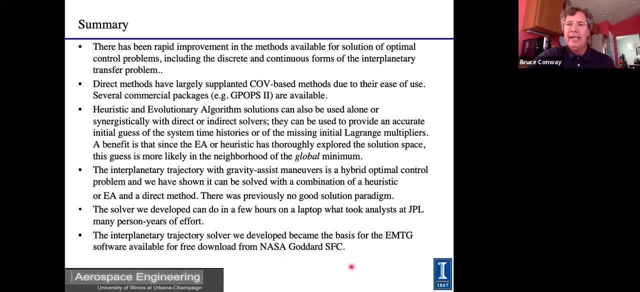 software with him. uh, they paid for it and it's now become the emtg or evolutionary mission trajectory generator, which is the software that nasa goddard now uses for all of its mission planning. it's been improved because he's had uh six years now to to work on it. uh, but it's you. 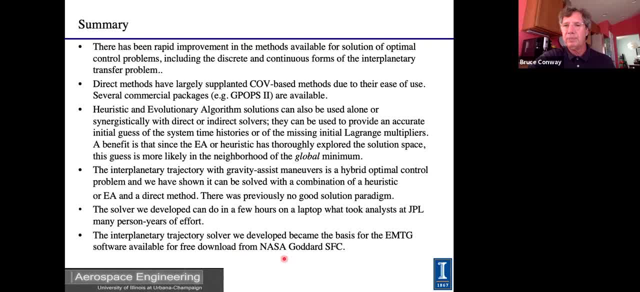 can download it for free from the nasa goddard space flight center uh website. i would mention, however, it's not, it's not what you call easy to use, but in it's free and if you work hard enough or put a phd student on it, uh, they will eventually get a solution with it. 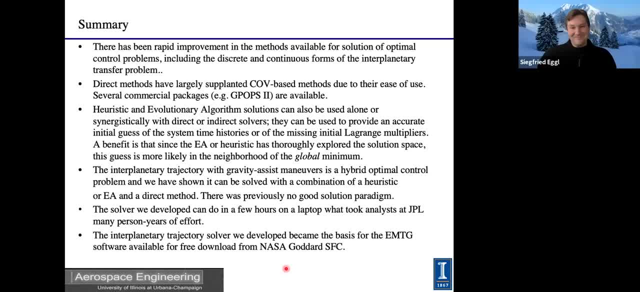 and that's, uh, that's what i have to say. thank you so much. um, thanks, bruce. um, if you want, you can unmute and clap and uh, since, uh, you are all still here, uh, i imagine, uh, you have some more time for for questions, and maybe bruce. 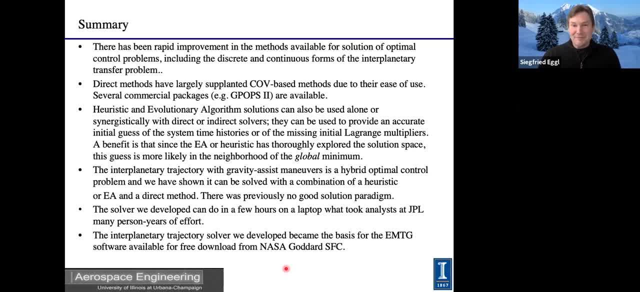 it's your break, so, uh, i don't know if you, if you're willing to answer a few. no, i'm no, i, it's fine, i'd be happy to answer any questions, sounds good. so what i would say is: um, raise your hand or, if you're quick enough, unmute and ask your question, please. 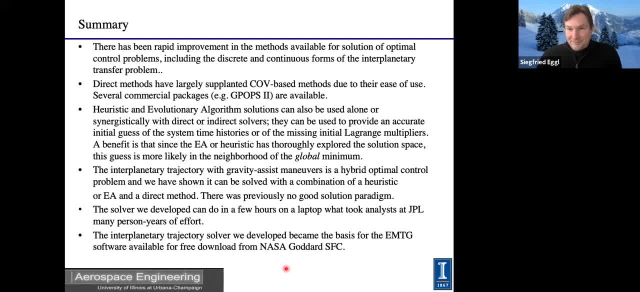 i don't see any hands raised, so oh yeah, um, daniela, please go ahead. thank you so much for your talk. it was very interesting. um, i have two questions. uh, first, i was wondering for your results about using the evolutionary algorithm for the trajectory to saturn. um, that, that several week. 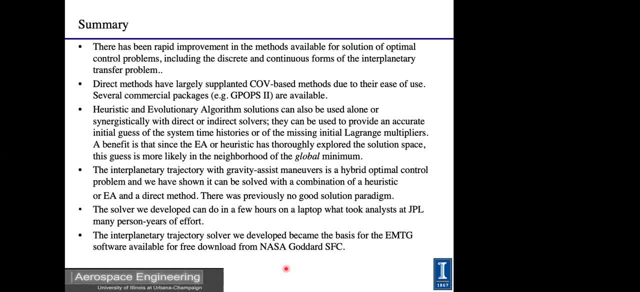 or month discrepancy that you saw at the end. did you try including the moon flyby and did that close the gap? or or you didn't try that? no, we, we didn't try it. we, we were, uh, we were pretty happy with, with, with what we got, and, um, that's actually a a fairly difficult constraint to to put into the. 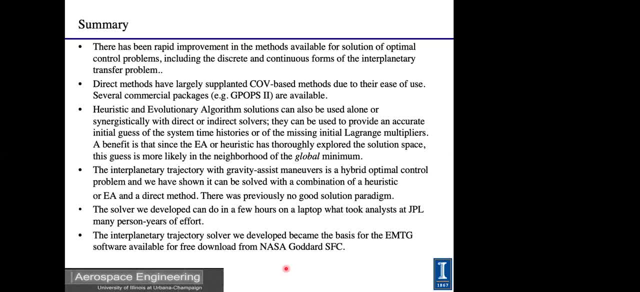 into the problem i see um. and the second question is: i know direct methods for things like low thrust trajectories have been criticized for the numerical issues dealing with the very small numbers involved in the differences in magnitudes of variables. um. have you had issues with them? and 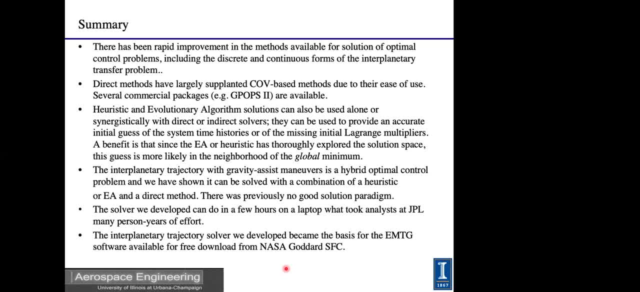 off the top of your head. what are some best practices that you've used? uh no, we haven't really had much problem. um what? what you generally want to do with these kinds of problems? the, the nlp solvers, are much happier if everything is roughly about the. 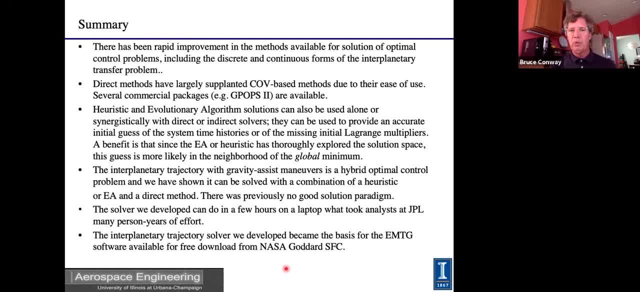 same order of magnitude. so if you try and work in kilometers and and um, days and so on, that's really bad. so what we always do is we work in normalized variables. so the distance unit is always one au and the time unit is that one year becomes uh pi time units and um. of course, the angle variable is: 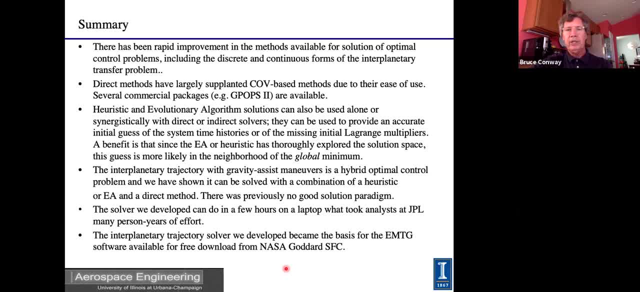 is trivial because it's just going between zero and two pi. so if, if you do that, everything is scaled except for the, the thrust, acceleration, um, everything is scaled to about order, uh, 10 to the zero or 10 to the one nychLo, and that that's if you, if you solve it, almost any kind of none, excuse me, non-linear programming. 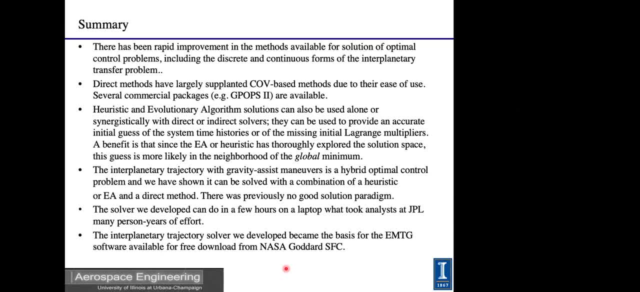 problem you, you find that that's what they pretty much always suggest- is to transcribe the problem so that everything's roughly the same size. okay, thank you very much and thanks for your work. question about actually, uh, implementing these orbits: so when you actually try to like, go run. 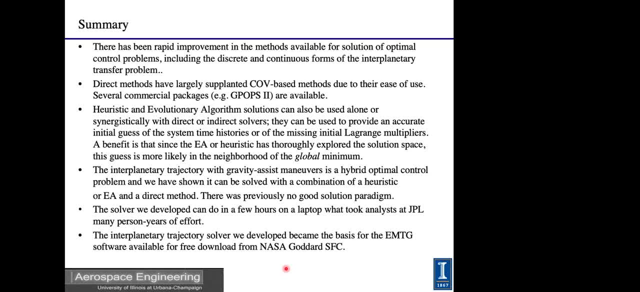 this: how accurately can you actually reproduce, like the trajectories that you've come up with in these simulations and you have to worry about, like, if this trajectory gets slightly off, um, how that'll propagate down the line? uh, i'm not sure if you're talking about, about solving- 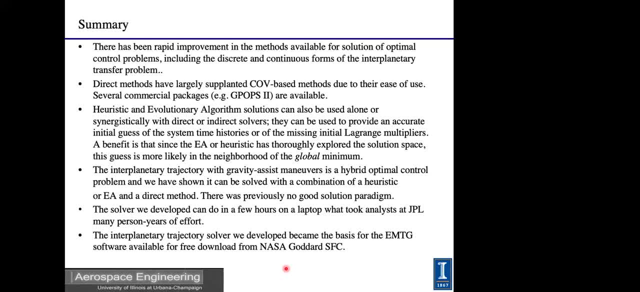 the trajectory, or actually flying it. actually flying it like, let's say, you burn or you end up like going slightly faster than you anticipated, or something like that. is that an issue that you run into? uh, well, not personally and not in my research, but, um, if, if you look at how jpl implements, 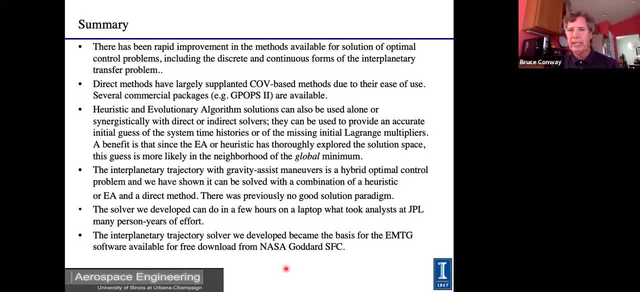 a flight. they're, of course, tracking the spacecraft, as, let's say, this recent one that's on its way to mars. they're tracking the flight and they have built in opportunities during the flight for doing course corrections, and so they will examine the the trajectory and if it starts to depart slightly from the 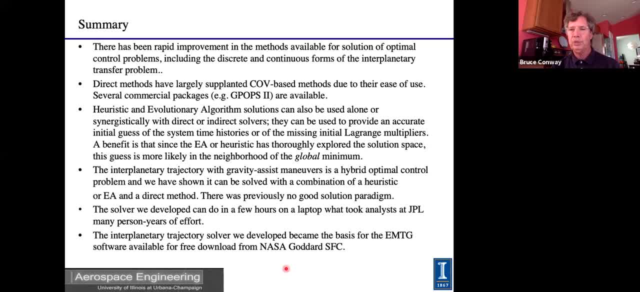 desired trajectory. they will, will do um course corrections at their specified times and in many cases the trajectory is so close to the projected, predicted one that they simply don't. they can simply uh bypass some of the um, some of the uh estimated course corrections, or even when they do them, they're they're trivially, trivially small. 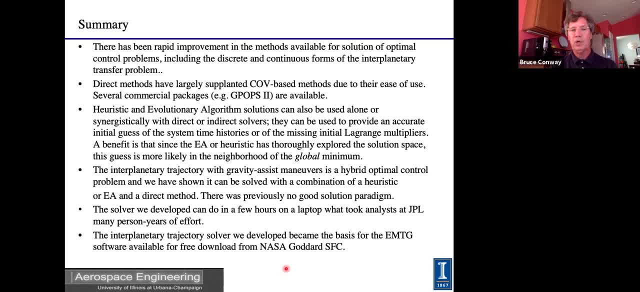 like you know, a handful of meters per second. so i guess what you could say is that they've developed the technology to a very high degree, um which of course you have to do if, if you're going to have a hope of landing, let's say a rover, within a you know, a couple kilometer circle on mars. 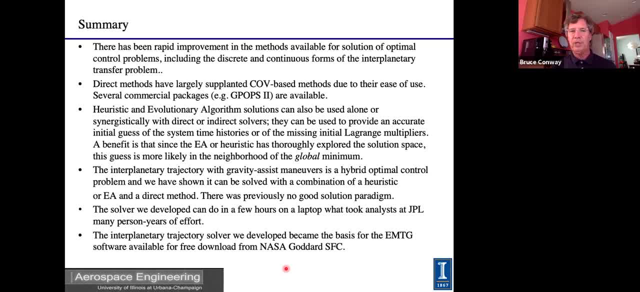 you have to know the location of that arrival point on mars in the solar system to that kind of accuracy too, right? so it's really incredible that the whole thing works as well as it does. don't jinx it, bruce. thanks, yeah, very interesting, okay. thank you, khan um, there's one more question. 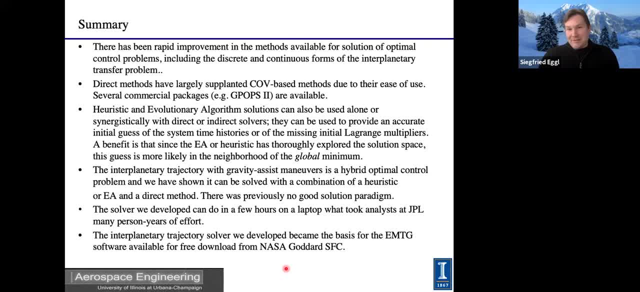 and then i think, uh, we'll let bruce have a quick break. uh, wes, please, thank you very much. yes, sir, thank you for your talk, and i just wanted to ask kind of a big picture question of where do you think this field is going as in, like, uh, what sort of questions are being? 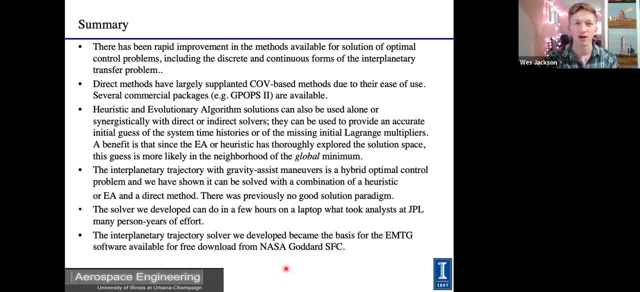 worked on right now, and what sort of problems do you see uh kind of on the horizon for your field? uh, wow, um, that's hard to say. when i started, uh, the available solvers, as i kind of alluded to at the beginning, were were not very good and they were challenging to. 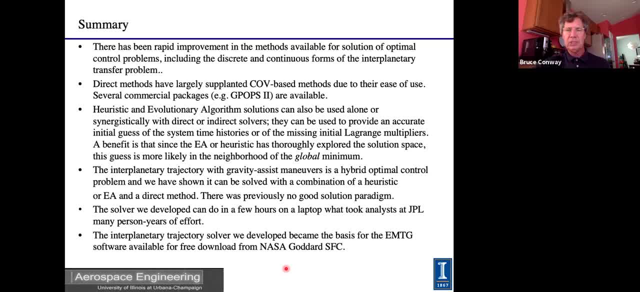 work with because you had to solve two-point boundary value problems. in fact, one of my phd student colleagues at stanford, working with the same advisor. he wrote his entire thesis and there's a long paper in the jay- guidance, control and dynamics. he wrote his entire thesis on a method for coming up with the initial lagrange multipliers. 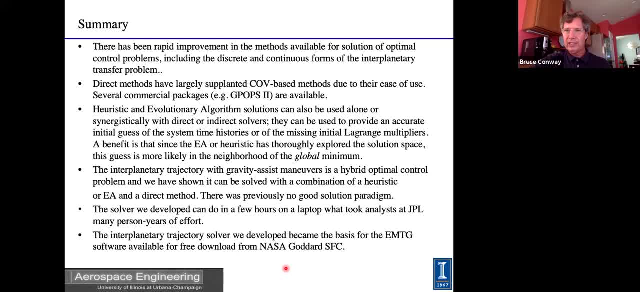 to solve that two-point boundary value problem for a low thrust transfer. that was how complicated it was. now it's. you could almost say that it's it's. it's relatively easy. um so, where is it going to go? i i think this method is going to be applied to more and more complicated problems. you're. 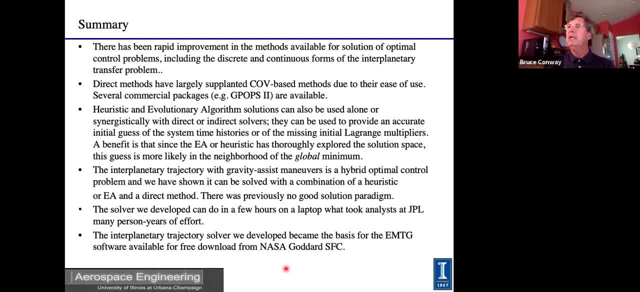 probably aware that one of the more challenging problems now in the last, oh, 10 or 15 years is, uh, leveraging these so-called invariant manifolds, which are these coasting trajectories in the three-body problem, okay, um, that allow a spacecraft to go from one point to another in either, uh, earth, moon, space. 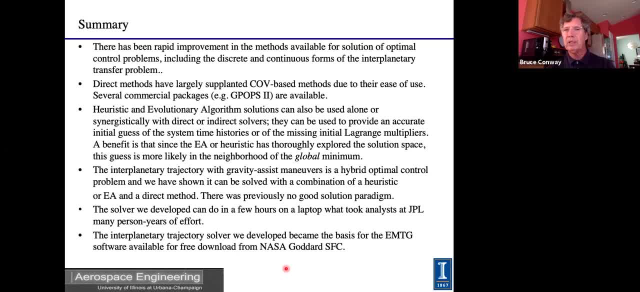 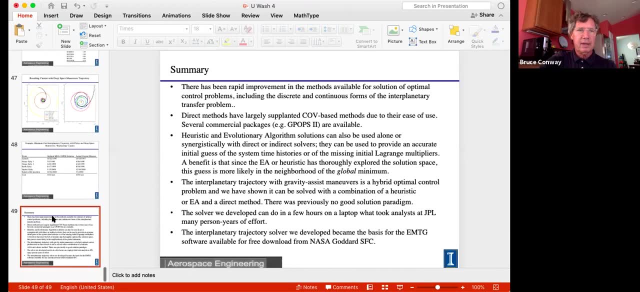 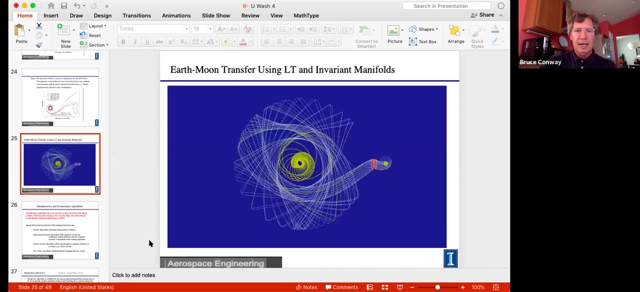 or even in the solar system, without using any propellant whatsoever. you, you can actually transfer from one invariant manifold to another. um, uh, let me see if i can zip, zip back here. uh, to the right slide this cartoon here. um, oh, right, right, uh, see if that's up. 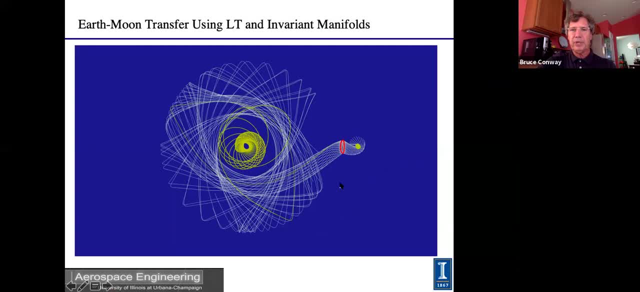 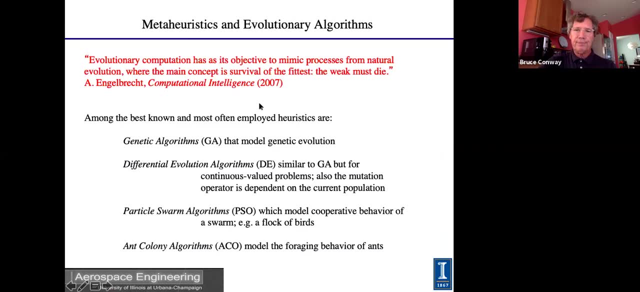 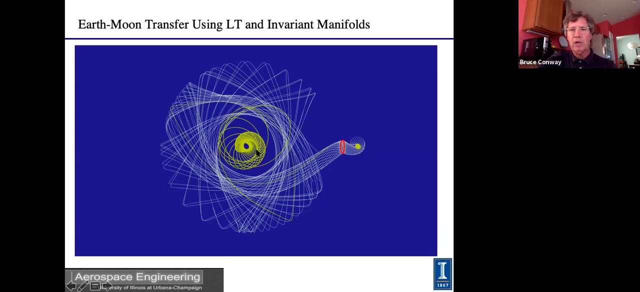 so this kind of thing? uh, this is an earth-moon trajectory using invariant manifolds, and when the yellow disappears in when the yellow disappears, it's not thrusting anymore. it's on one of these invariant manifolds and it doesn't look like it because this cartoon is in a system that's rotating with the earth. 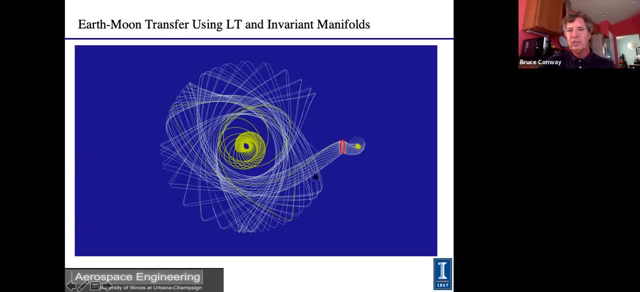 moon system, but you can kind of see it here, this thing that looks like a fishnet stocking. these are possible invariant manifolds, meaning coasting trajectories that would allow a spacecraft to go, when the thrust is cut off, and arrive and even enter this halo orbit about the. 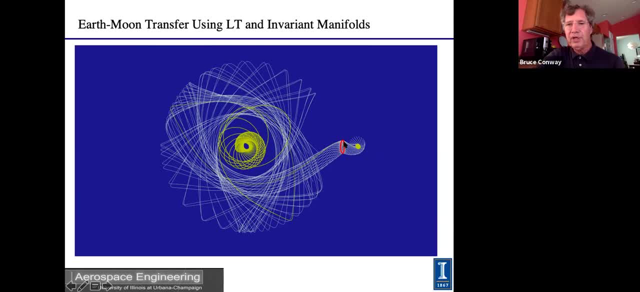 interior lagrange point and then with a trivial delta v, like just one or two meters per second, you can hop off of that and get on a trajectory that goes to the moon with no further effort. it actually goes close to the moon. so you can't use these for man missions because they take way. 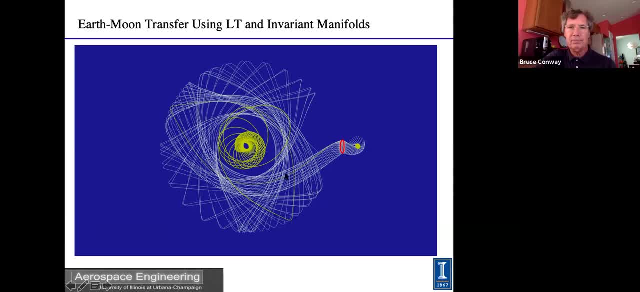 too much time. but if you simply want to send, like um supplies to a lunar base, you could do this. so this is a very active field, using, uh, this kind of trajectory optimization to do these trajectories that use both thrust and invariant manifolds to get places with very low cost. 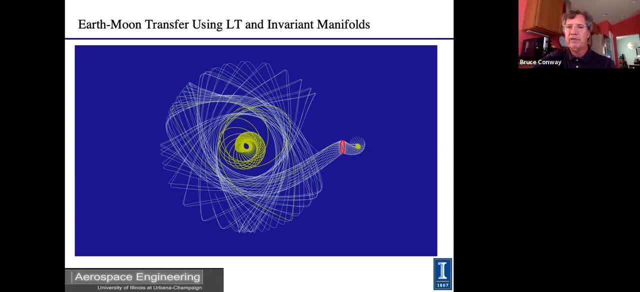 compared to the way that we did it say during apollo, or that's invented, envisioned for the, for the upcoming the artemis, yeah, yeah, Beard, that's probably the the most uh dynamic application for this kind of work that's going on right now. that's the most challenging problem that that there is right now. 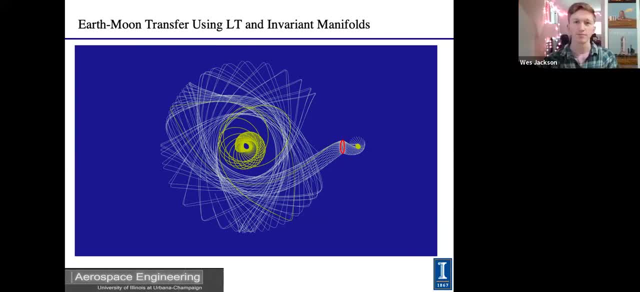 well, thank you right. thank you very much. i think we'll leave at least five minutes for Bruce to take a breath before he is meeting with with James. thank you so much, everybody, for coming sure. If you have any more questions, I'm sure Bruce would be happy to answer them through email.